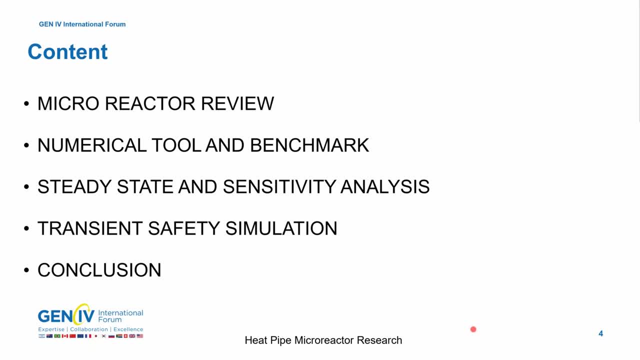 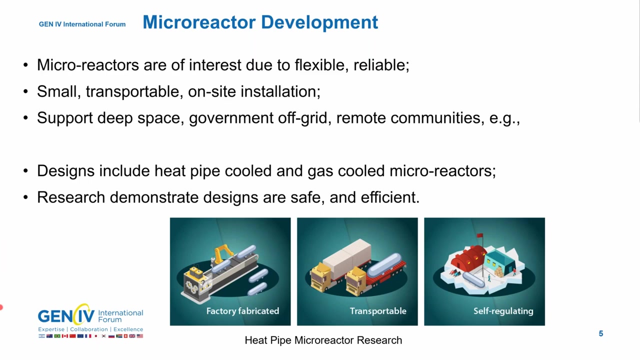 the heat pipe microreactor. So first of all I would like to go through the development of microreactor history and to introduce some basis concepts of how heat pipe works. So microreactor is becoming very popular, becoming more popular and attracting more interest due to its flexible and its reliable. 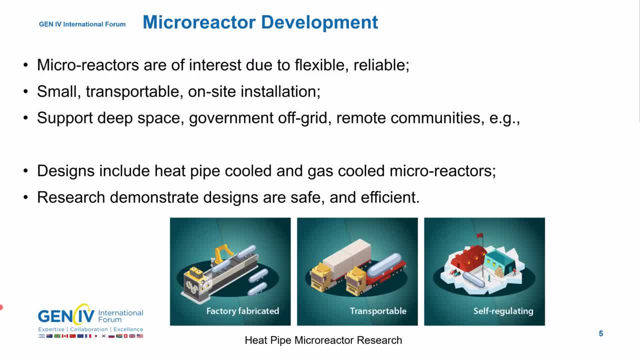 power supply And it's small enough, could be transport and provide onsite installation And it has been applied or could be applied in multiple application situation, For example, the explanation of deep space, the garments and off-grid energy supply, and also energy supply for some remote communities. 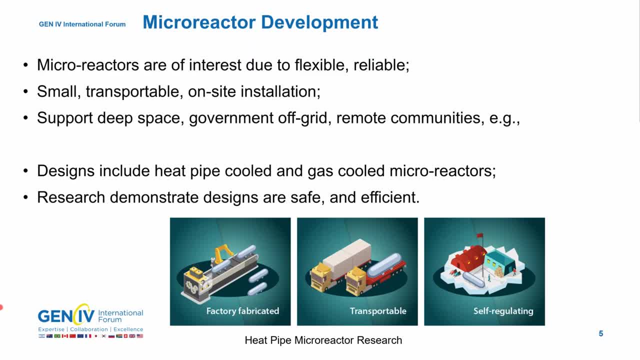 And currently the most popular designs mainly includes a heat pipe-cooled micro-reactor and also the guys-cooled micro-reactor And, however, last year, a lot of concepts and technologies are not tested or not proven, So we still have to conduct the research to demonstrate the designs are safe and efficient. 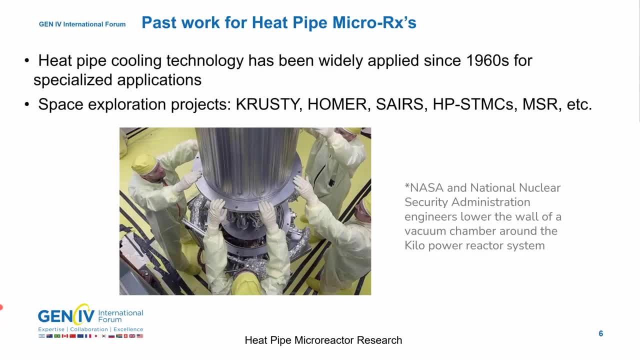 enough. So efforts developing the micro-reactor technologies could start from 1960s, along with the using of nuclear energy, And a bunch of projects like Cluster, Homer and a lot of others are already being conducted. Starts from 1960s, and this figure shows an example of engineers from NASA and the National 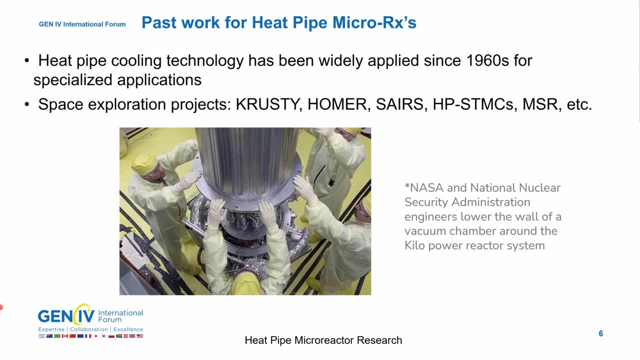 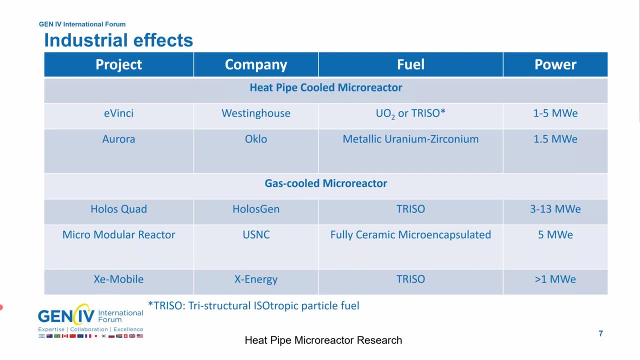 Nuclear Security. They are working on a kilopower reactor system. The efforts are still going on. So I list some of the current efforts from the United States industry. So, for example, the Westinghouse is working on Eric and Okra from California is working. 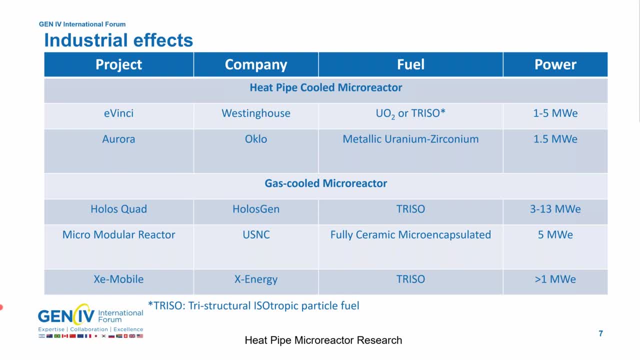 on Nona, And both of them can see the uranium as a fuel and the Westinghouse also can see the diesel fuel. The reactor power is between one to five megawatts And we also have other efforts from the gas-cooled micro-reactor. 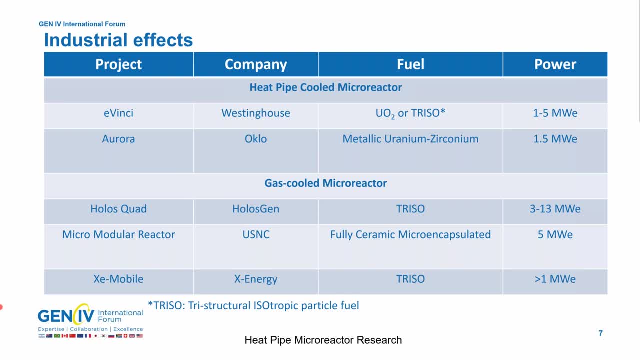 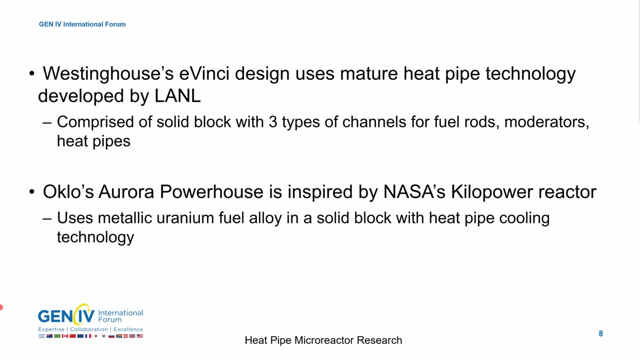 So the companies like Hologens, USNC and X-Energy are working on it And most of the power are below 15 megawatts- And a bunch of the details of the heat pipe micro-reactor design. So Westinghouse Eric did then use the Mitra heat pipe technology to build a nuclear reactor. 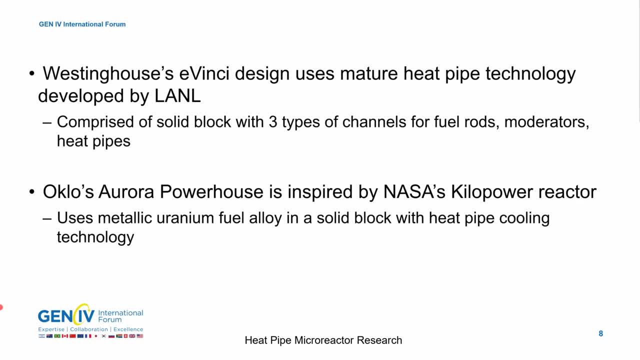 And then we also have other efforts from the gas-cooled micro-reactor. So the companies like Hologens, USNC and X-Energy are working on it And most of the power are below 15 megawatts. And we also have other efforts from the gas-cooled micro-reactor design. 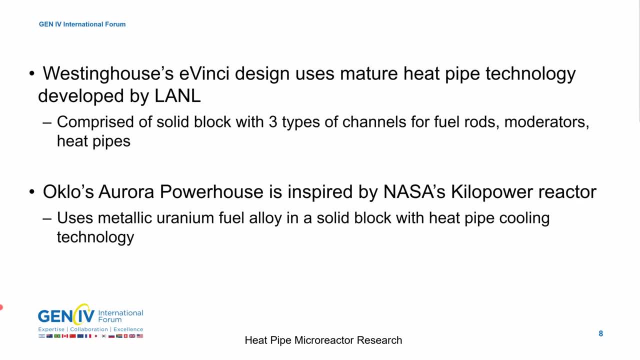 So the companies like Hologens, USNC and X-Energy are working on it And most of the power are below 15 megawatts. And we also have other efforts from the gas-cooled micro-reactor design, So the Jenny's micro-reactor design. 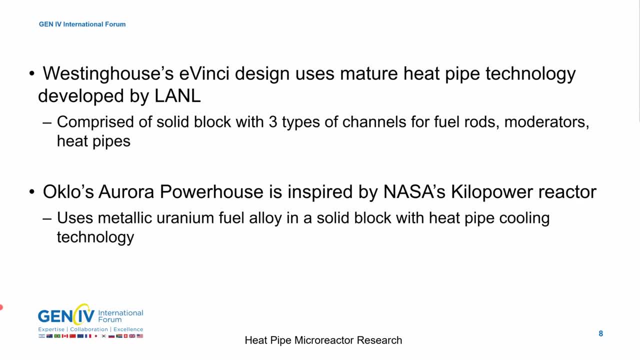 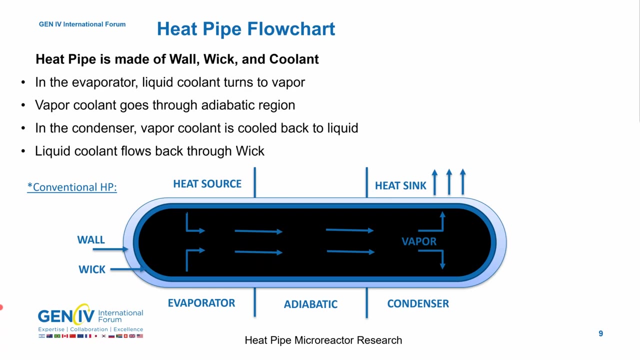 And so now let me open this and just …. Emily Jen, from the plant it is connecting to the cluster, like I think from the File seem here. And another background I would like to share is how the heat pipe works. So I see in this figure, from internal to outside the heat pipe could be separated. 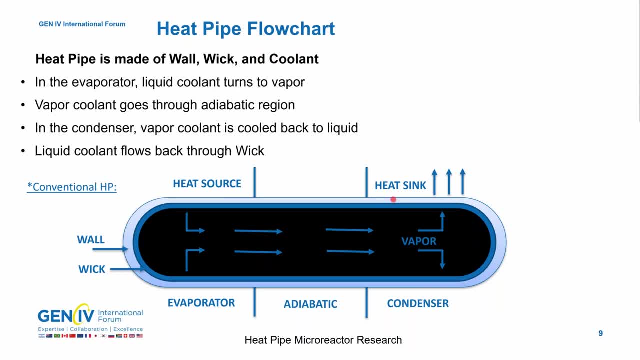 into three parts: the current, the weaker and the lower, And from the left part to the right part. the heat pipe also includes three parts: evaporator, adiabatic and the condenser. So firstly it's liquid sodium here at the current trainer of the left side. 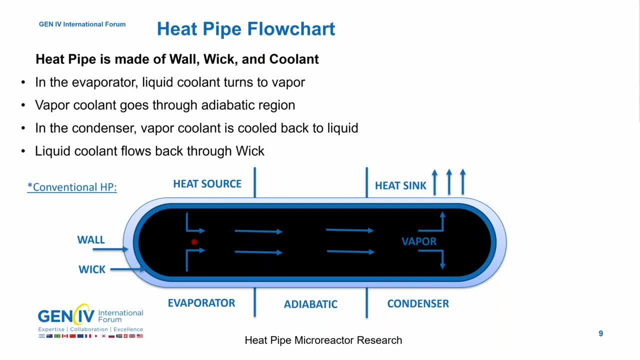 And here the liquid solid will be heated into vapor solid and go through adiabatic and go into condenser. Heat will be cooled down into liquid sodium again and flow back through the weaker, So slowly, this process. the energy will be transferred from the heat source to heat sink. 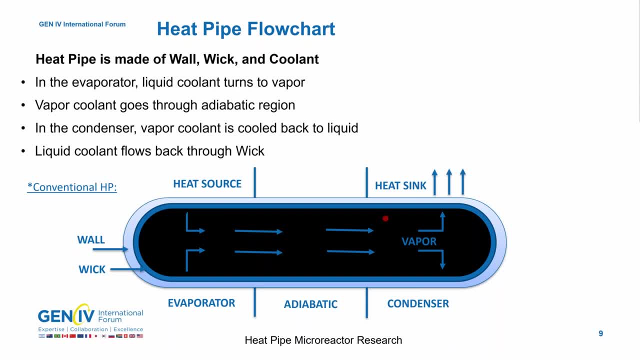 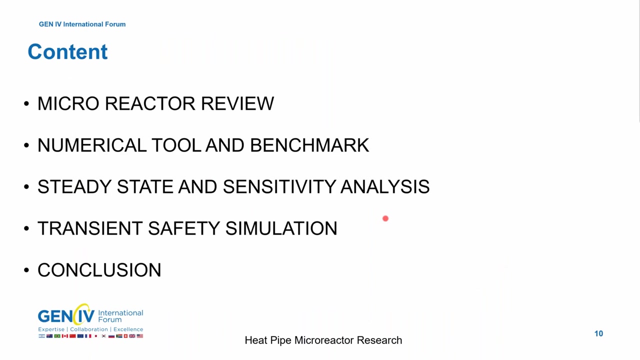 and the process doesn't need extra energy supply And the energy transfer coefficient is high. That's why heat pipe is so popular and it's considered to be a pride in micro-reactor technologies and also a bunch of multi-industry engineering application. So in first chapter we introduce some background of the micro-reactor development history. 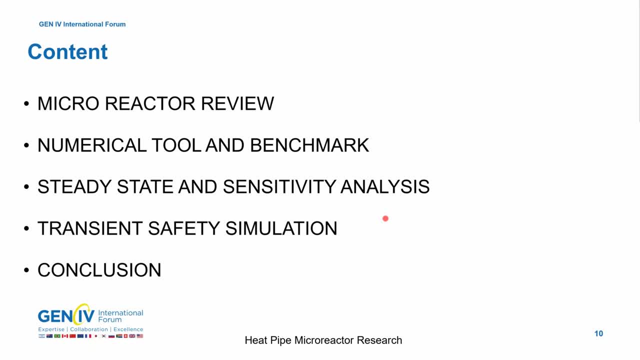 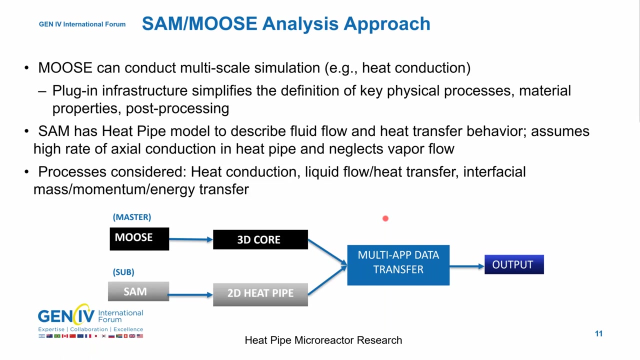 and then we introduce How the heat pipe works And then after that, I would like to introduce the numerical tool we are using and the benchmark comparison between our results and Argonne National Labs' results as part of verification and validation. So the numerical tool we are using is called SAM and the MOES. 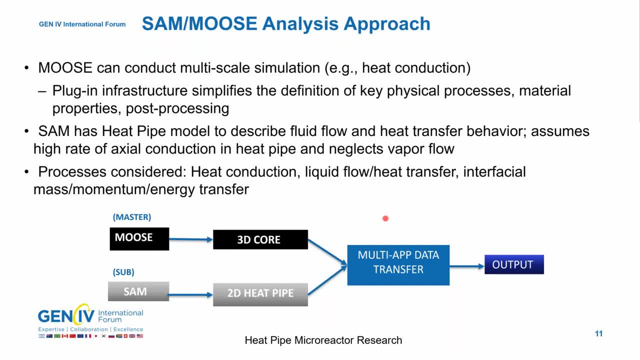 And we also use cherries and qubits to build the geometry And the mesh for us. SMOOTH is a multi-physics platform originating from Idaho National Lab. It can provide definition of key physical processes, material properties and poster processing. 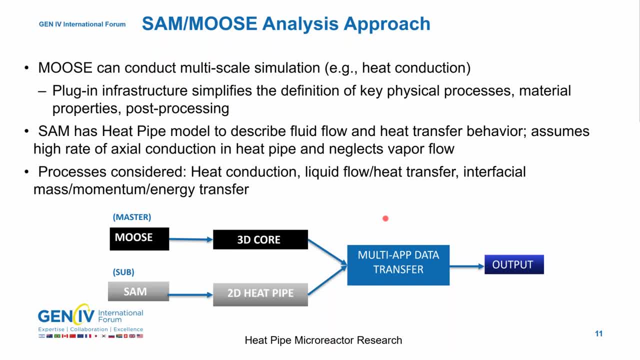 CHERRYS and Qubit is the software from Sandia National Lab. It can provide the building of CFD geometry and also meshing. So SMOOTH can read the 3D geometry from CHERRYS and Qubit. And STEM is a software prepared for the advanced reactor and it's origin from Argonne National Lab. 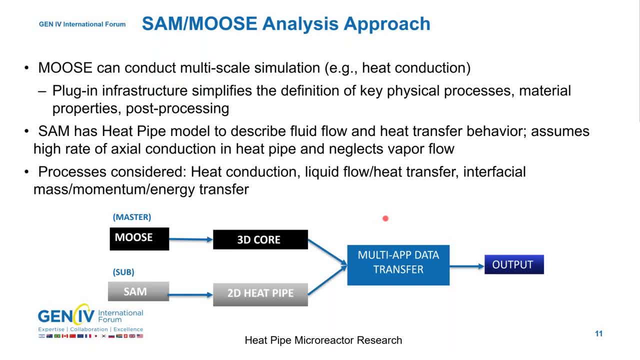 And STEM also has a 2D heat pipe model which can transfer, which can calculate the fluid flow and heat transfer behavior in the heat pipe. So the whole process could be summarized either 3D heat conduction, liquid flow, heat transfer in the STEMS model and interfacial mass momentum. 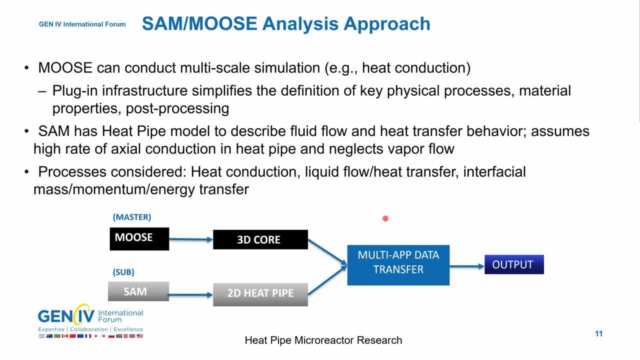 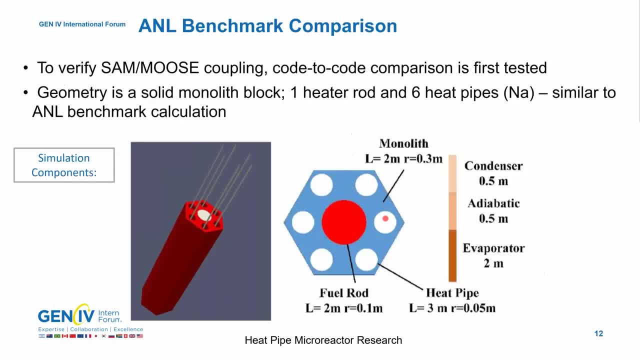 and energy transfer in a heat pack model instead. And the following feed explain how those softwares are working together. And here is the benchmark example problem provided by Argonne National Lab. So at this moment, since we don't have any published experimental data, 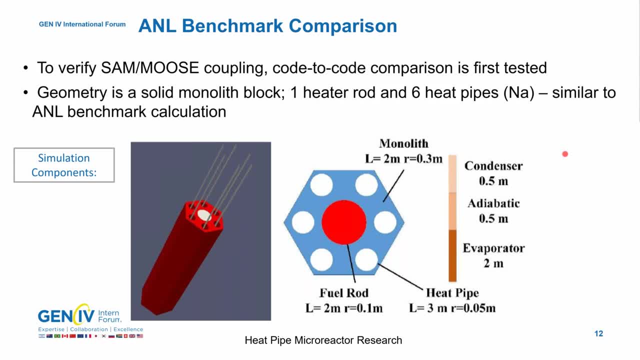 we have to do a code to code benchmark comparison to check our calculation result. So, as we can see from the left figure, so the red block is the model list and the inter-cylinder is the filler And there are six heat pipes insert into the model list. 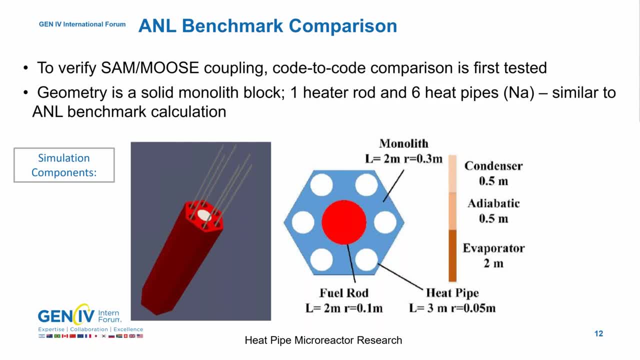 And the right figure is a cross-section from top view: Filler, heat pipes, MPD for 2D heat pipes and model list. The filler and the model list is two meters as an assumption here And the heat pipelines is three meters. 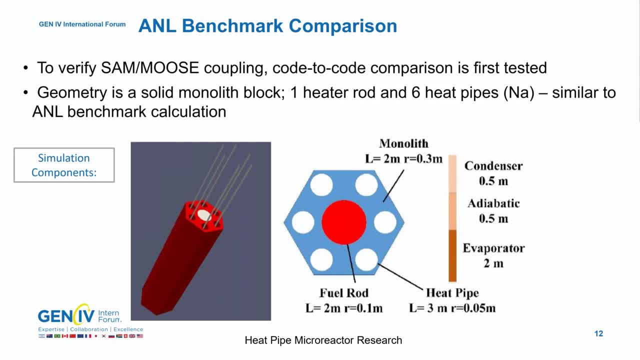 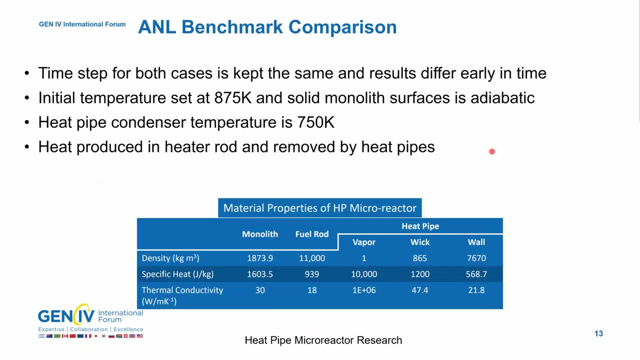 while evaporator is also two meters. It's totally insert into the model list. And we also have an ideal and the condenser. They are 0.5 meters each And we have some other details, parameters for the design. So, first of all, we keep our. 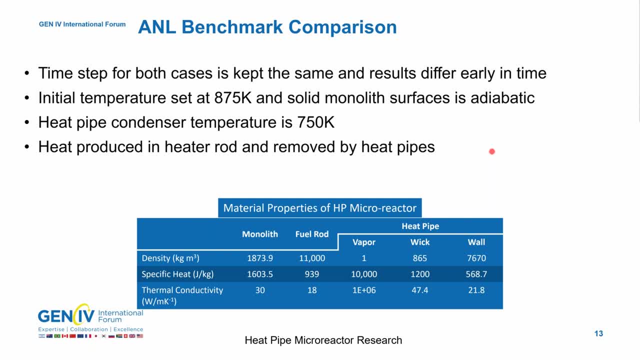 time step for both calculations there. And the ignition temperature for the system is 875 Kelvin And the solid model list boundary condition is ideal bedding And the heat pipe condenser temperature is 750 Kelvin. The system energy source is the electrical heater and the energy sink is the heat pipe. 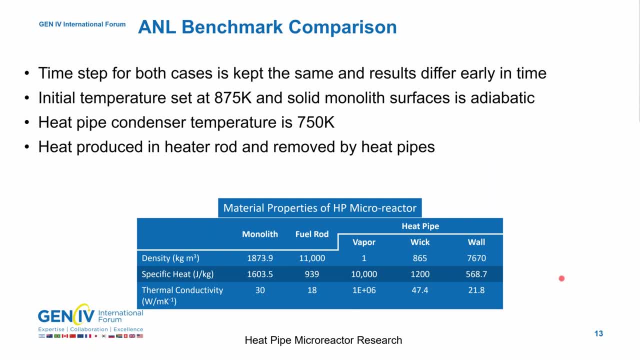 And in this table we list a bunch of thermal properties, Including the density, specific heat and the thermal conductivity For the three parts of the system: model list, fill rods and the three components of the heat pipe, Including the coolant, the weak and the warm. 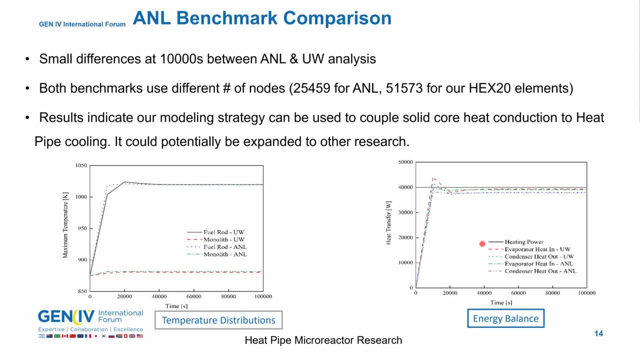 And we come to our result. So left figure shows the maximum temperature comparison And the right figure shows the heat transfer comparison. So we can see that the results of UW and Argonne National Lab match each other very well. Lastly, a few very small difference between these two model. 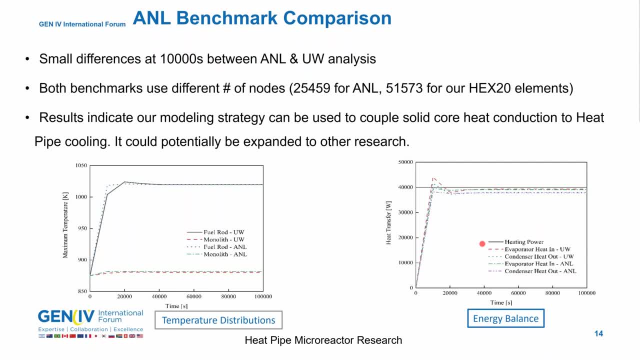 It's the mesh nodes, So we are using different software to build the geometry And the number of nodes are a little different. Lister here. We assume that's a reason for a small difference at 10,000 seconds And also at least 10 point is a transfer. 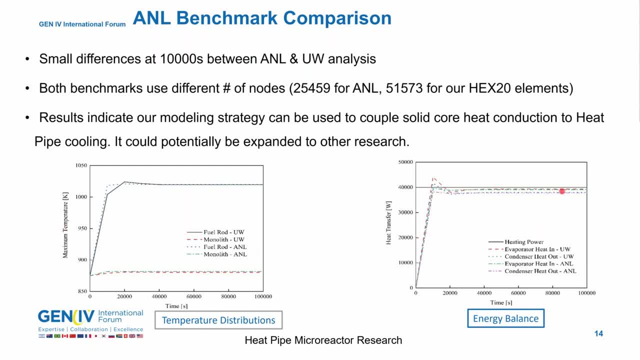 from a temperature increasing, heat transfer increasing comes to a steady state. So we still believe that our calculation results matches to Argonne National Lab's results well, And the code to code benchmark comparison could support our future numerical answers for the safety transient check for the heat pipe micro reactor. 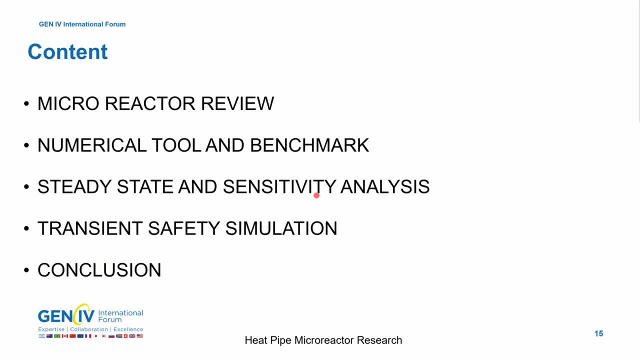 So, after the introduction, background information of the numerical tour, and then a benchmark, verification and validation, we start to do a state-to-state calculation And, based on the state-to-state calculation, we selected a few critical parameters to check our sensitivity answers. Check how these critical parameters affects the result. 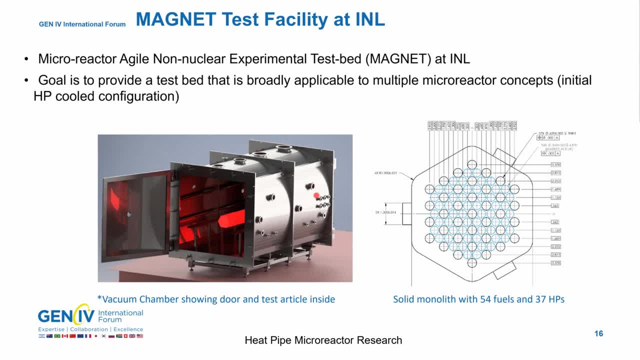 The research target we selected is called MAGNET. The full name of MAGNET is Micro Reactor Engine, Non-Nuclear Experiment Testbed And it's a facility at Argonne at Idaho National Lab. And this facility it's a testbed. 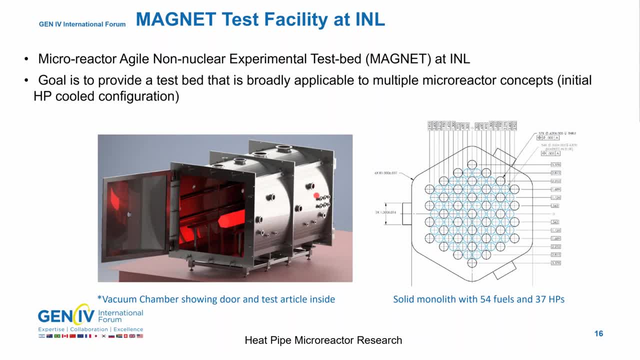 and it's open for different micro reactor design. So ignition design is a heat pipe code configuration And the details of the design are shown on the right figure. So we have 54 filters. It's the blue circle And the black circle is the heat pipes. the number is 37.. 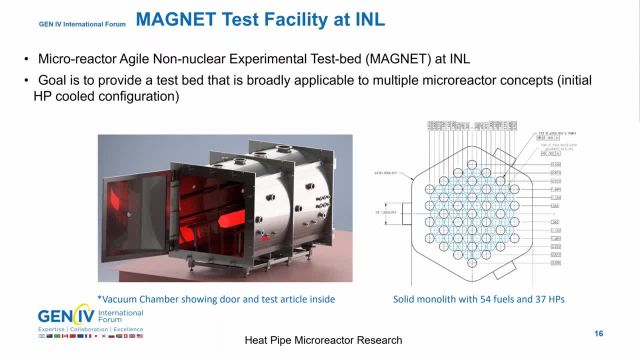 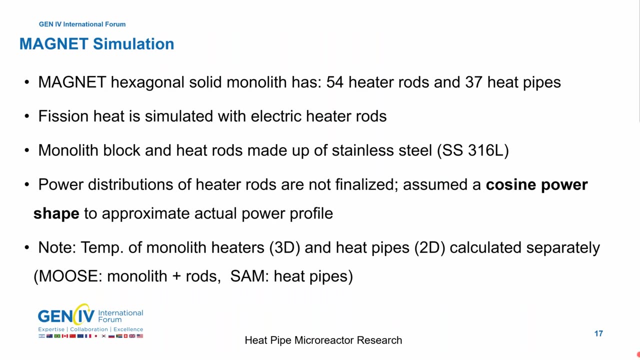 And here left part is the figure for a testbed And it's MPT internal And when we have the experimental facility ready we can insert it into the testbed And a bunch of more details of the experimental design. So the total value of the trainers are 91.. 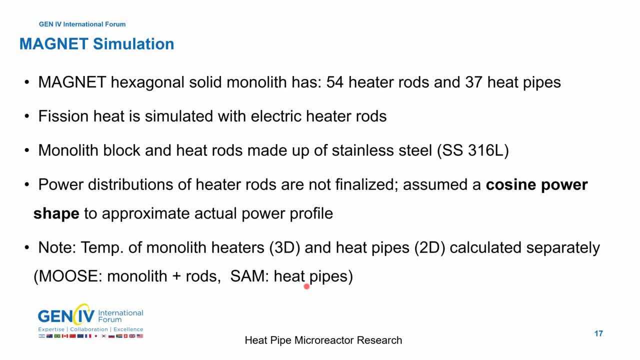 And the energy source. the system is heat by the electrical heater And the monolith block, and the heater is made of stainless steel. So we know, in reality this design could be some material difference, like monoliths could be graphite and the filters could be uranium or trisophilic. 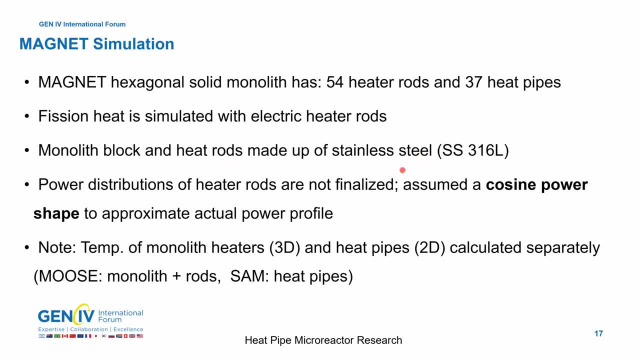 For experimental design. we use stainless steel here. And for the power distribution. at the initial flow calculation we can see all the power in different fuel are same. That means, in other words, we didn't consider the enrichment of the fuel because we had to use the new fuel. 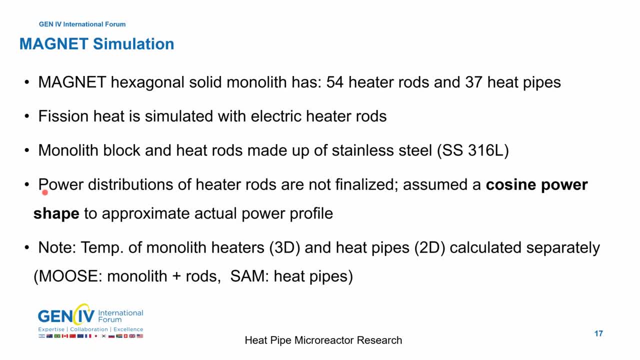 But in the future we can consider the industry suggestion and maybe we'd reduce the power At the deciding. an increase the power in the center of the monolith And then each of the fuel we assume a cosine power shape which is closer to actual power profile. 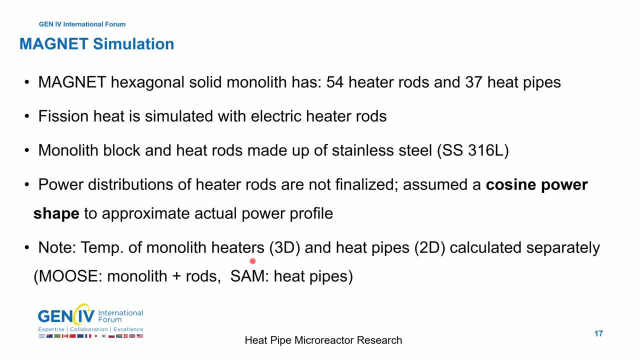 And then the important note is that we calculate the 3D monoliths and electrical heaters. electrical heater and we calculated a 2D heat pipe. They are calculated in the same time and same system, but in two different parts of the software. 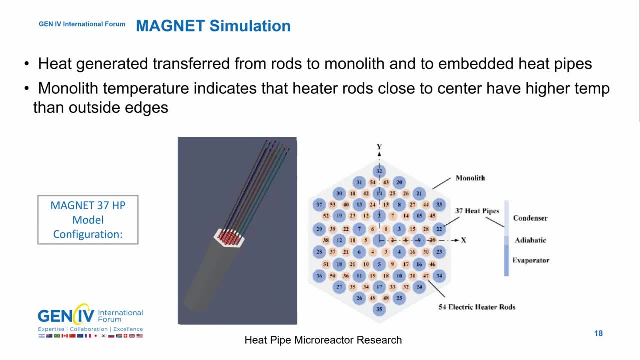 Okay, so here comes our model of the magnet facility. This is the 3D model including the model list and the filters, the heat pipe inserted. So it's very similar to our first example, but it's more complete And the right figure shows the cross-section from the top view. 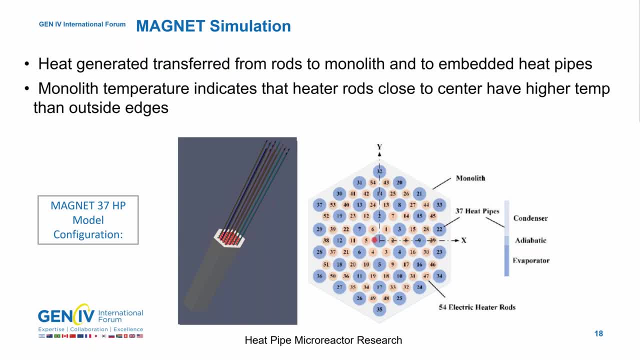 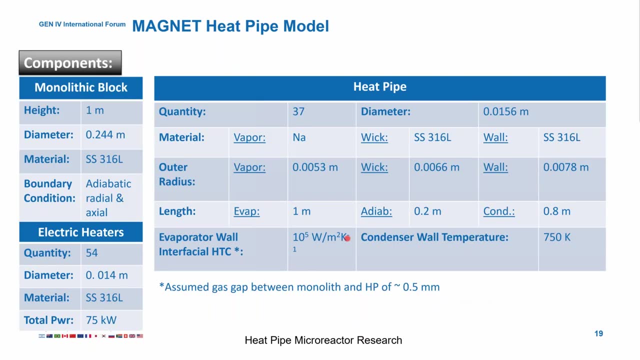 And here we are also an order of heat pipes and the filters in different number. So this could help us explain the calculation results much better in the following result And here are some more details of our experimental facility. So three most important parts: model list, electrical heater and heat pipe. Model list: head is one meter. 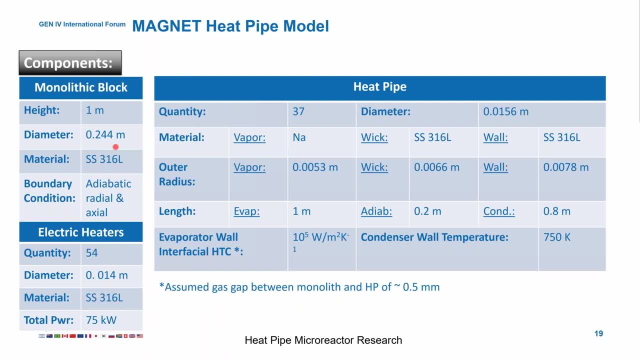 Diameter is 0.244.. Material is stainless steel, Boundary condition is idiomatic, The electrical heater number is 54.. Diameter: 0.014.. Stainless steel and the power is 75 kilowatts. So this power is connected to the number of heat pipe. So we assume each heat pipe could. 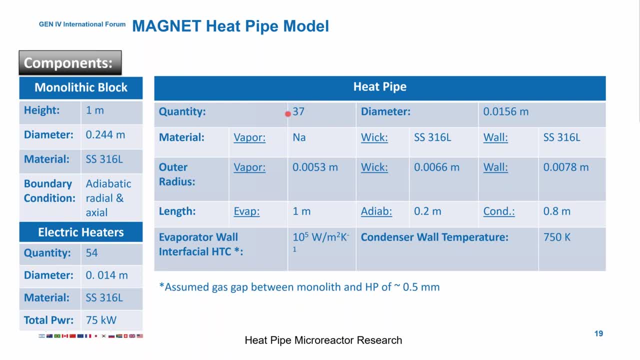 remove the power of two kilowatts and we have 37 heat pipe. And that's why we define the power, total power, At 75 kilowatts here And diameter of heat pipe is 0.0156.. And the materials? the current is sodium. 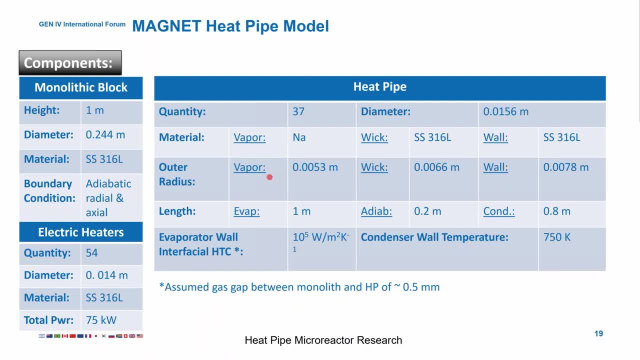 weak and the water is still stainless steel And the radiance is increasing from current to weaker and to work. The lace is two meters total, One meters evaporator- same to model list- and electrical heater And 0.2 meters idiomatic and 0.8 meters of condenser. 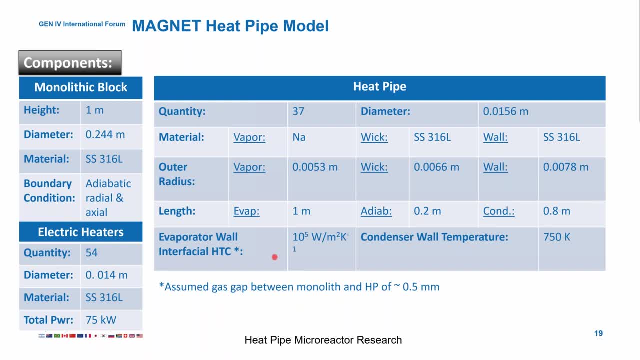 And the heat transfer coefficient between the model list and heat pipe evaporate part is 10, 5 megawatts per meter square per kilowatt And the condenser wall temperature is 755 kilowatt. So this is the details of the magnetic facility. 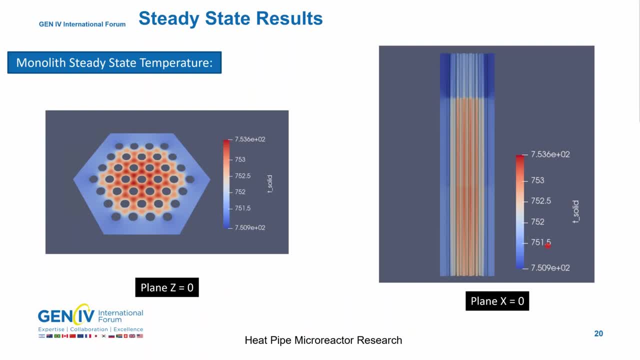 And once we put all this information into our numerical modeling we can get the results, And the most significant results we can get is the 2D temperature distribution. We use the software called pilot view to deal with the results. So this is the results of the base. 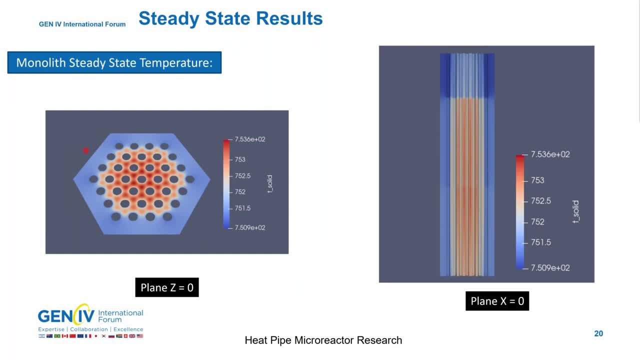 steady state results And we can find the list is the cloud section from top view and cloud section from side view And the temperature. here there are some significant hot part is the location of the fuel and the modulus between each fuel is also hot and we leave empty holes for the 2d heat. 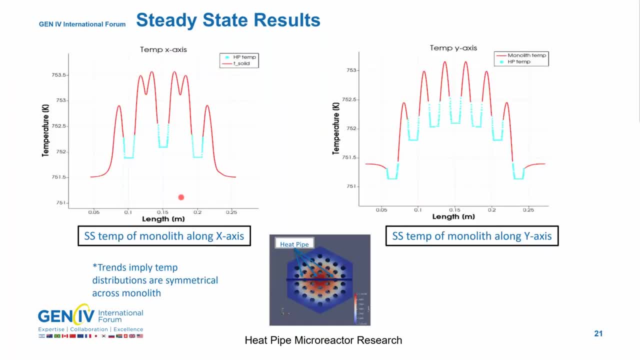 pipe and besides the 2d temperature distribution cloud, we can also use grapha to get our result. for example, so you can see, we selected a line on the surface of a cross section of the modulus fuel and heat pipe system and we can show the temperature history: temperature distribution. 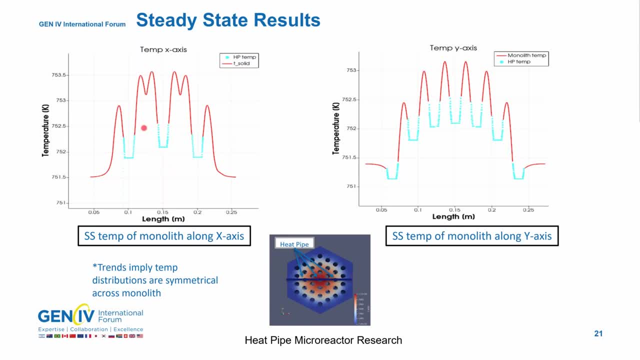 along with this line at x-axial. so the peak point are the location of the electrical heater and the low point is the location of feed pipe, and the temperature between them is the modulus, and when we connect all the temperature together we can find it's a constant length. 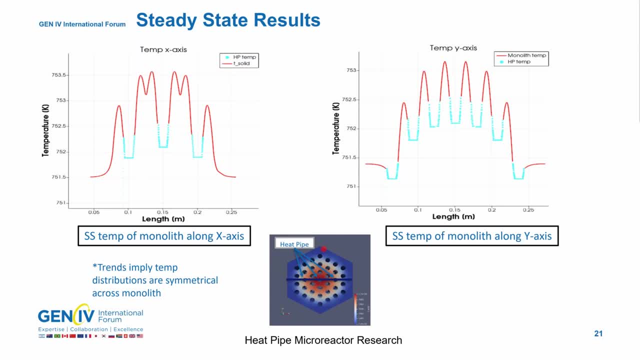 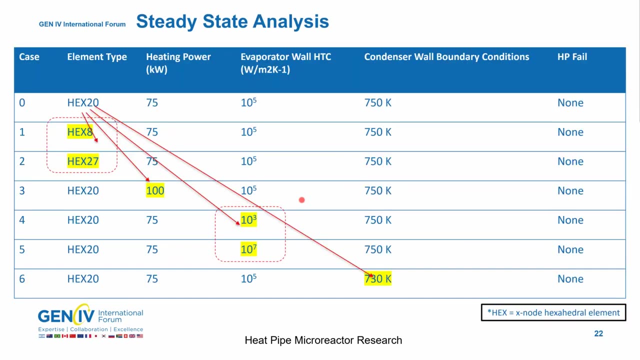 and we also can draw a figure from y-axial and we draw these figures. is trying, we draw these graphs is trying to help us and find the location of hot part in the system. and after the steady state we did a bunch of other different change of parameters to compare the sensitivity answers. 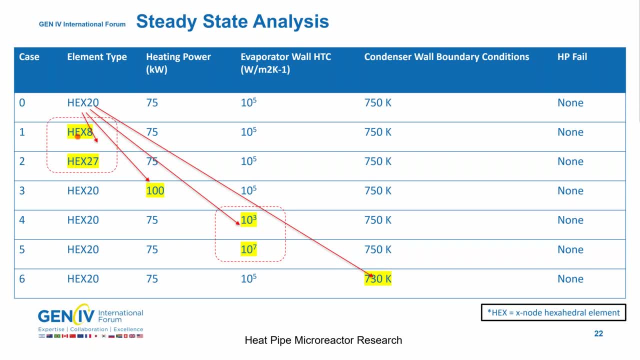 so in first group we change the mesh type. initial mesh we are using is hx20 and we can change it to hx8 and hx27. another parameter we change is the heating power. we increase it from 75 to 100. and the third sensitivity parameters is the heat transfer coefficient. 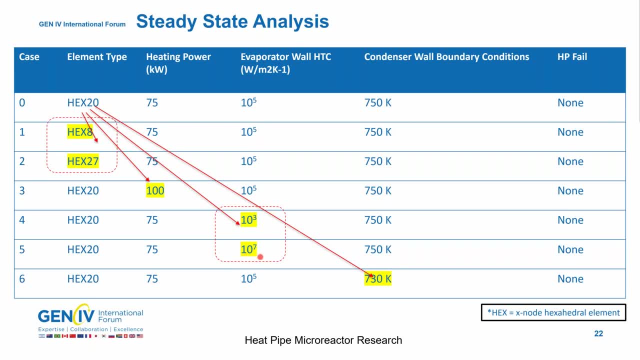 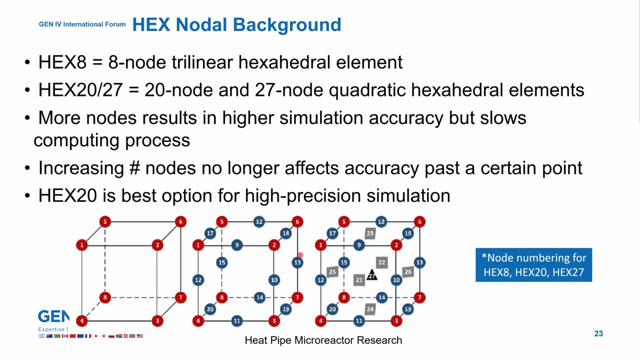 we transfer it from 10: 5 to 10: 3 and 10: 7, and the first one is the condenser temperature from the heat pipe and we change it from 70, 750 kW into 730 kW and some of the background information of what's the mesh type. so hx8 means eight nodes. 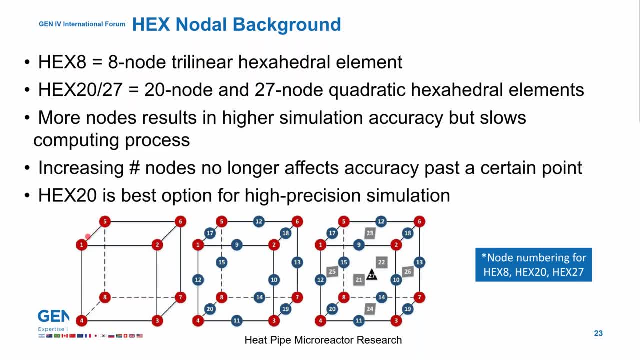 so when we want to describe a volume, we use eight nodes to describe it, and the hx20 and 27 means 20 and 27 nodes. So, in theory, when we are using higher number of nodes, the calculation result, the prediction, is more accuracy. However, since we are using more source to model it, 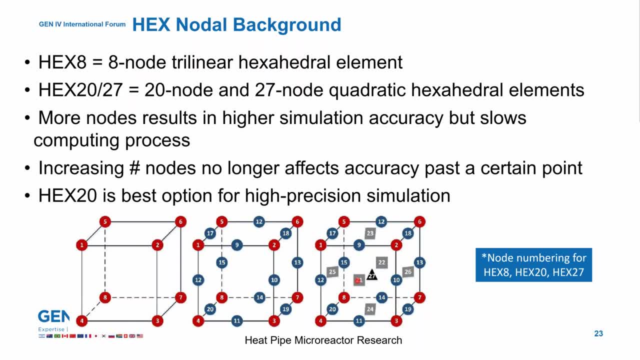 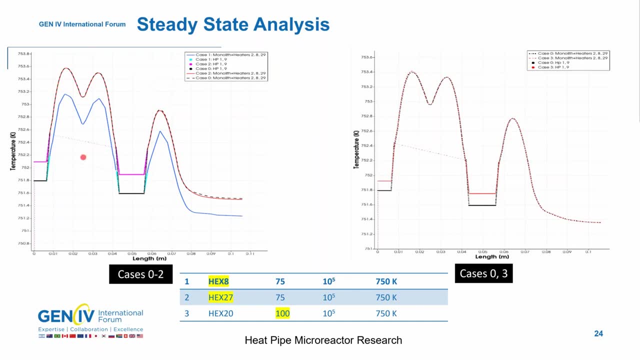 the calculation speed will be delayed. So we have to balance the demand on the prediction and the accuracy calculation speed. Then it comes to the result. The first one is comparison of different mesh types. So we can notice like maxX20 is the land here if we reduce the nodes. 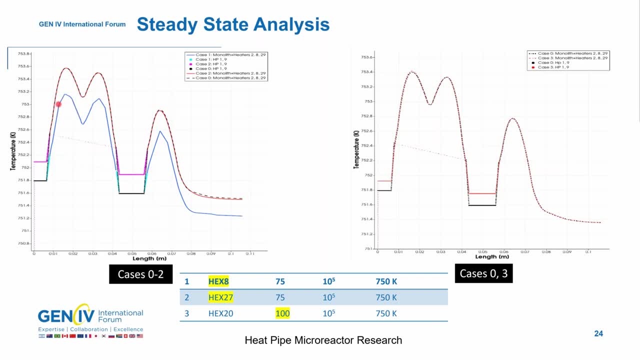 number reduction is changed And there are much fewer points in the land. of course the accuracy is lower If we increase the NOS number from 20 to 27, the result is not changing too much, which means HX20 is. 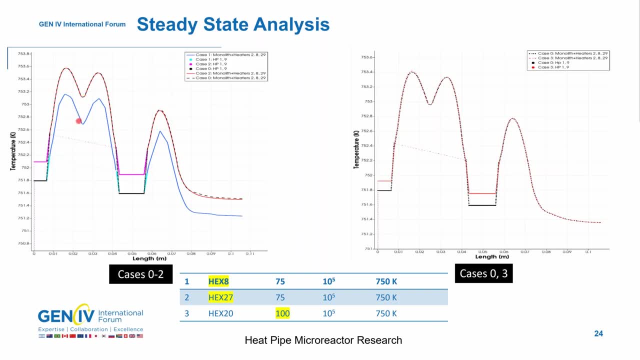 our best option. We don't want to delay, reduce it to reduce the prediction accuracy. We also don't want to increase it to reduce the calculation speed. We also check some other parameters like heating power, And we can find, with two different heating power, the heat pipe still. 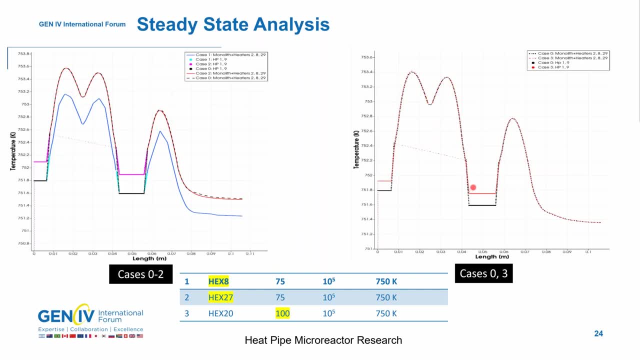 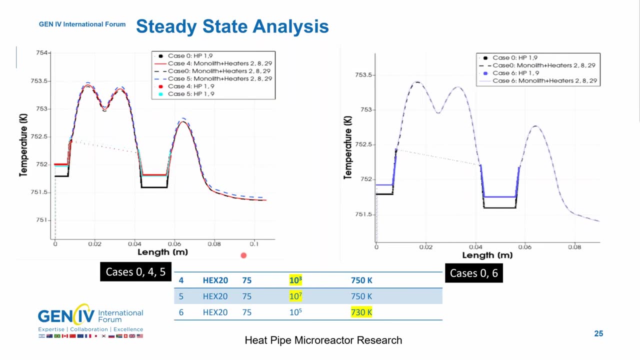 works very good. It transfers energy out very efficient and the APF model temperature are not changed too much. We also change the heat transfer coefficient to the left figure and also the condensation temperature of heat pipe at the right figure. Of them the modulistic and 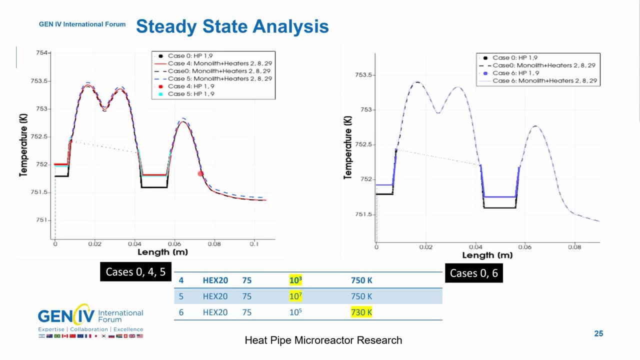 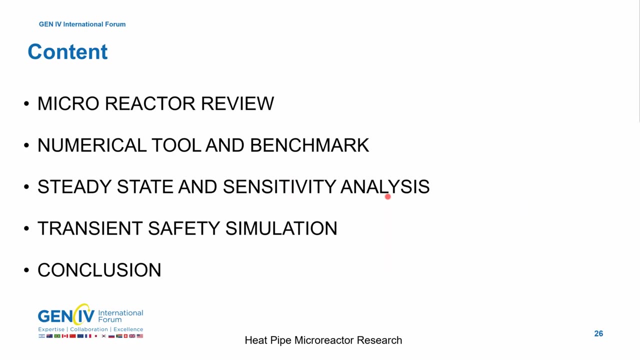 field temperature is not too much So, which means all these parameters are under the limit value of the sensitivity test. So in section three we introduced our work on a steady state and also a test of the sensitivity for different numbers of parameters, And after that we start to think about what we can do. 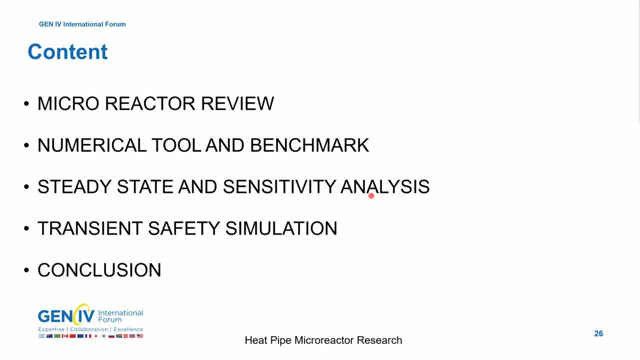 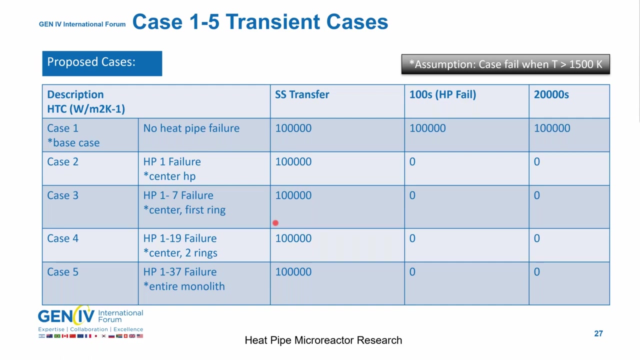 for some transient safety case. What will happen if different numbers of heat pipe fails or heat pipe fails at different time? So we want to check the integrity of the heat pipe micro reactor in some transient case. The first group of the transient is listed in this figure, So case one is the base case. 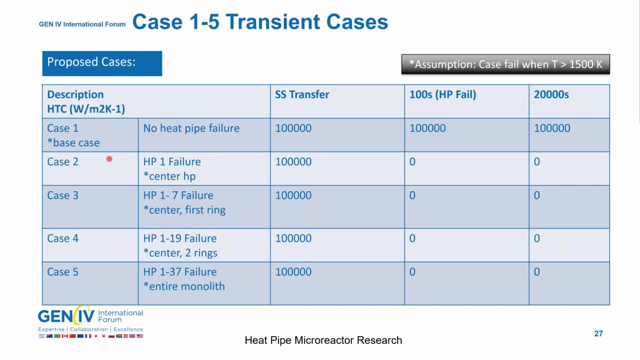 no heat pipe fails And in case two, as we discussed before. so we have four rings of heat pipe. So in case two, the first ring of heat pipe fails. Case three: first two ring heat pipe fails, Three ring heat pipe fails And four rings all heat pipe fails. 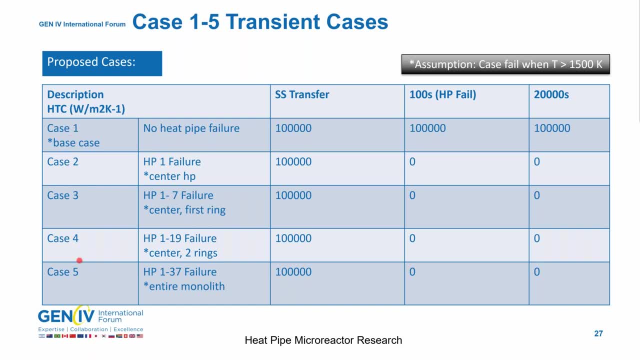 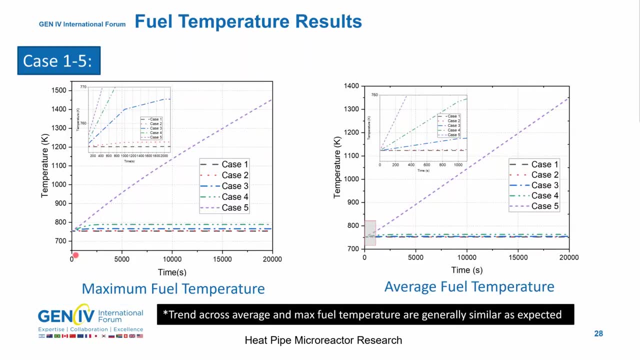 That's the difference between case one to case five in the transient safety calculation. So in case two, the first ring of heat pipe fails. Case three, all heat pipe fails. And then we come to the calculation results. First result we want to check is the maximum. 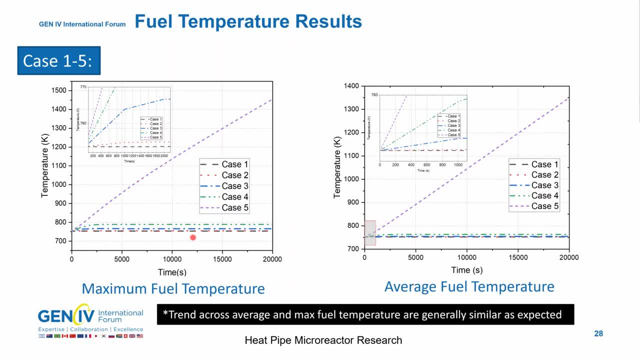 and average field temperature. So as we can see here, the pink line when all heat pipe fails, the temperature increasing to super high, which is over 1400 Kelvin, almost 1500 Kelvin. So it's much higher comparing with the melting temperature of stainless steel. 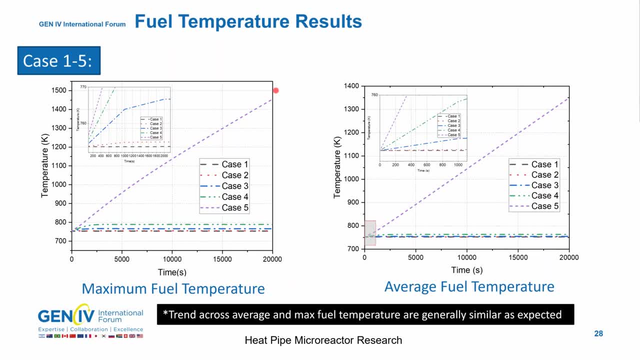 And of course it's later in the integrity of the heat pipe micro reactor system. And at the same time we can compare the other calculation result And we can observe that when more heat pipe fails, the temperature increasing could be much higher, Speeding. 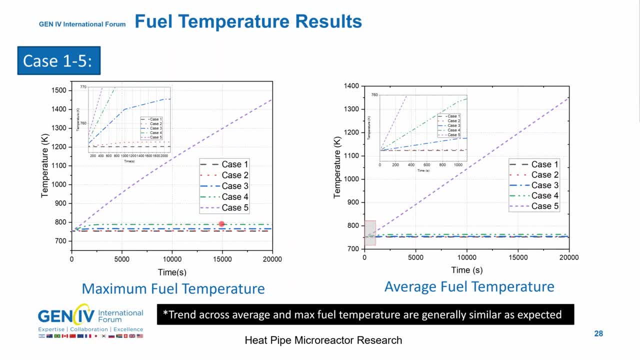 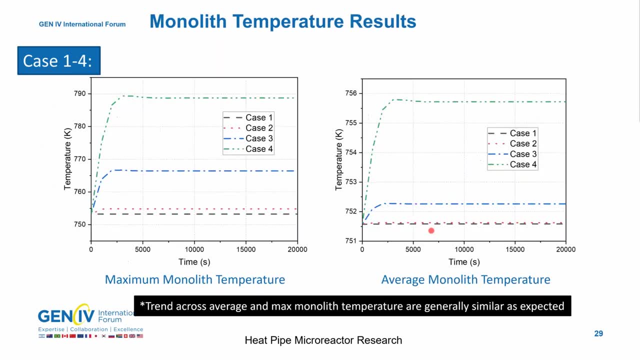 could be much higher And the final temperature is also higher. The same situation is observed in the figure for case two And we can also check the average field temperature And we also check the peak and average modulus temperature And in these two figures we get rid of the crazy pink line. And here we can find that. 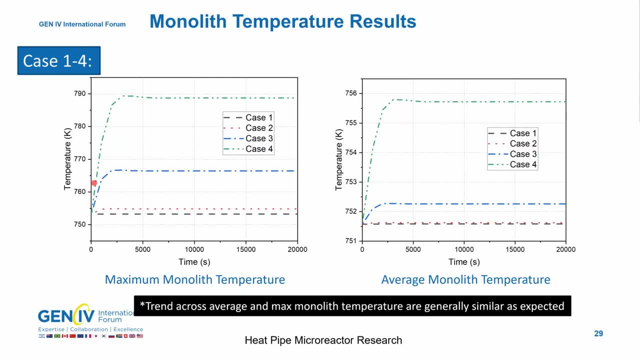 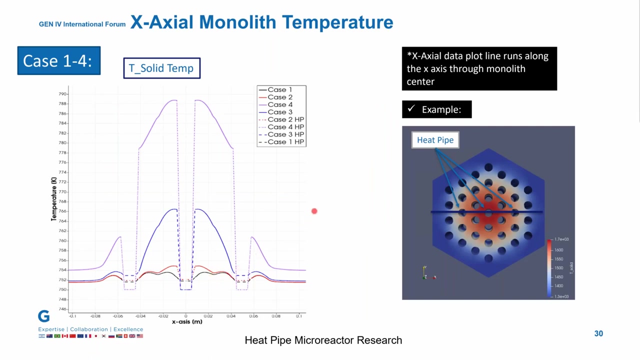 again the temperature. when more heat pipe fails, the increasing of the temperature is much higher and also the final temperature could be higher. comparing with different arcs And the tendency is in different parameters- no matter it's maximum or average model is temperature And another parameters we can compare is the temperature distribution at this line on the. 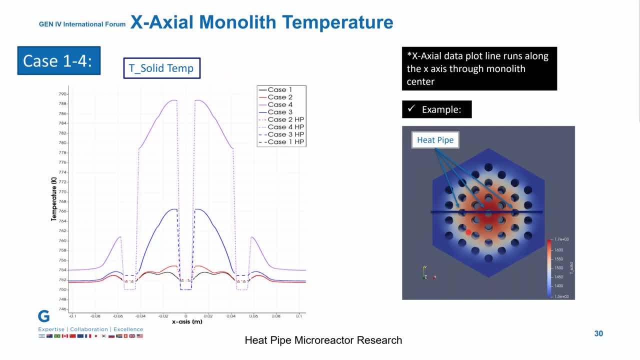 surface of a cross section from top view And we can clearly found a comparison from case one to case four and the peak point is the location of heat pipe. a peak point is location of fuel and the low point is location of heat pipe And the connection is in the model is 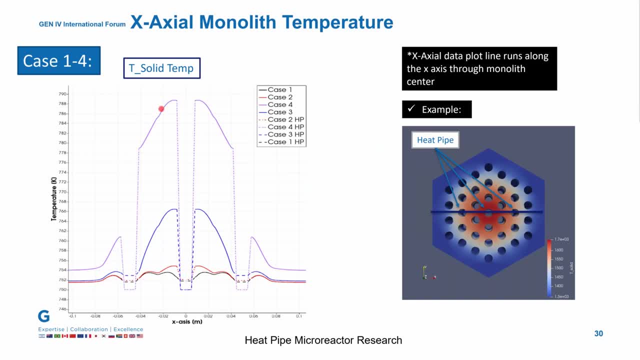 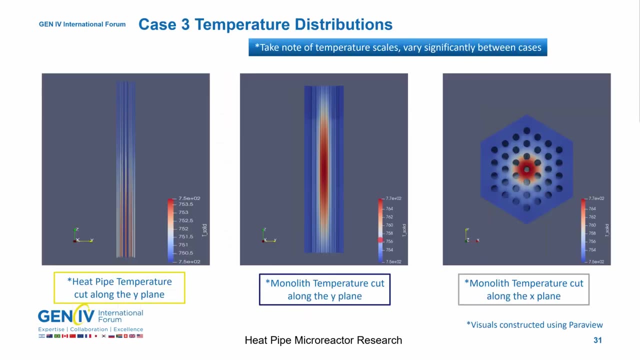 and we can still clearly see like well, heat pipe fears, high temperature, UVO though. So this is three ring fears, two ring fears, one ring fears, and the black line is the steady state. We selected the two case example to show the temperature 2D temperature cloud. So 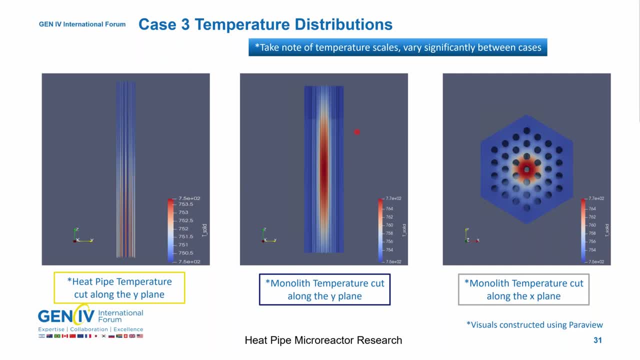 these three figures are heat pipe. model is from side view. model is from top view. So for the heat pipe we can found a red parts are in the bottom. So we can find the red parts are in the bottom. So for the heat pipe we can find the red parts are in the bottom. So we can find. 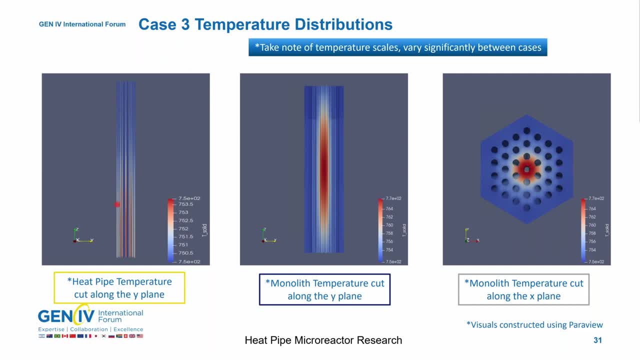 So where the heat pipe is inserted into the model is, And the center temperature is much higher, And the cloud wheel from side could be something like this, And the temperature distribution is similar to a cosine distribution, which matches the definition of the fuel power. 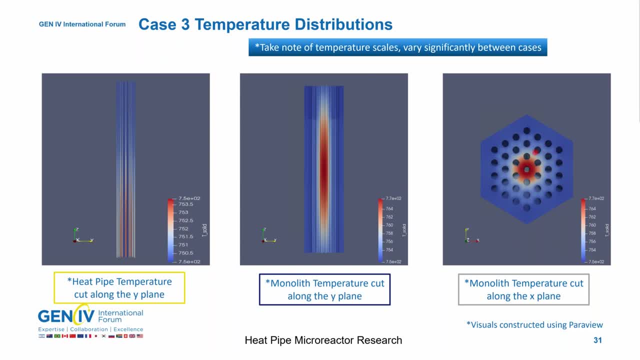 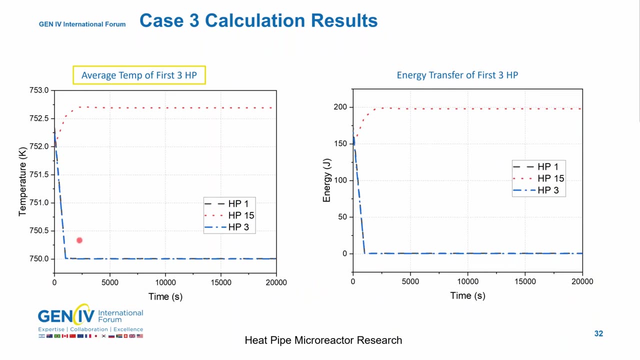 and ignition condition. And also we observe a similar thing, the 2D heat pipe distribution here, And we can also check the values of the heat pipe. So we already discussed the light, the heat pipe in ring one and heat piping ring two. first, 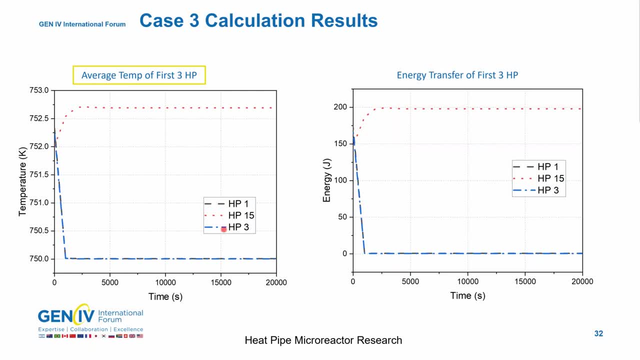 And here we observe that heat pipe one, heat pipe three in ring one and ring two It will force to the bottom, same to the condenser temperature, 750 Kelvin, And heat pipe 15 is from ring three And that's why it's still. 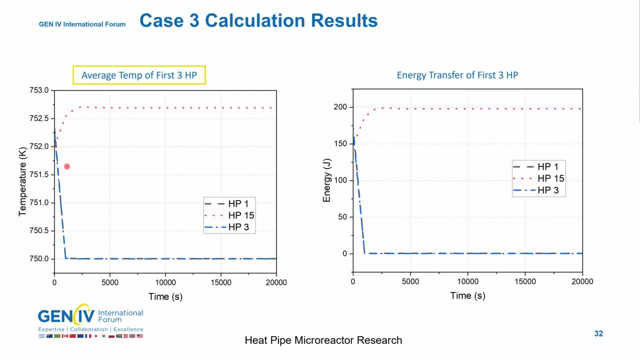 still working And when some other heat pipe fails, the bottom of heat pipe of ring three increase to transfer more energy from the system And the energy transfer of the three pipes it matches the situation we observed for the temperature. Another case is case five. 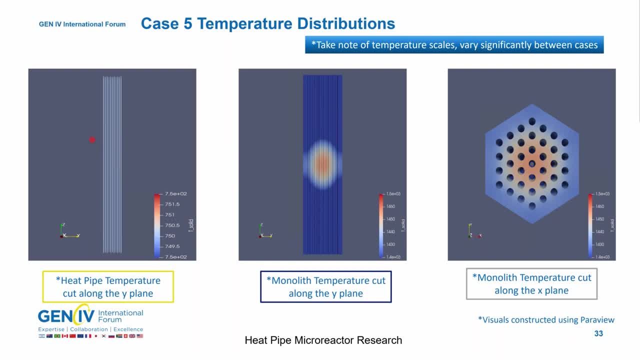 In this case all heat pipe fails and that's why the 2D heat pipe situation. temperature here doesn't make any change. And also we check the model is temperature from side view, from top view, and we can observe light. If we compare the color, it's over 400 Kelvin. 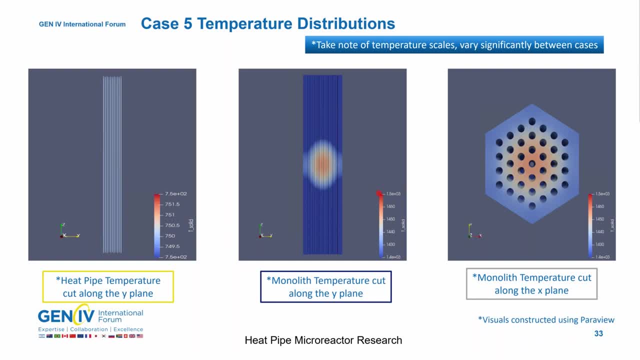 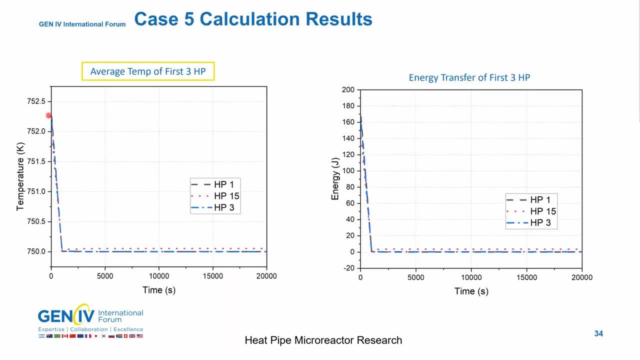 below 1500 Kelvin. It's super higher, higher than the maintain temperature for a stainless steel And also for the situation of heat pipe. everything force down means all heat pipe failures. And the last: there's not any heat energy transfer from the system. 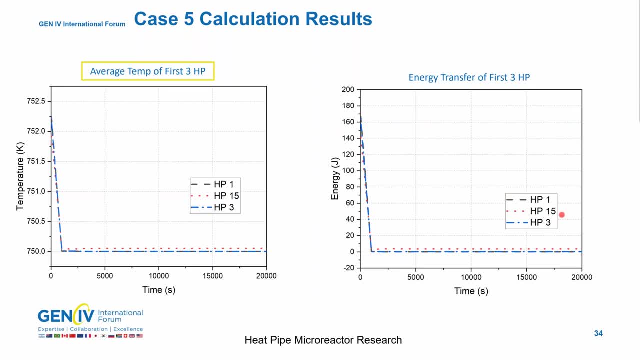 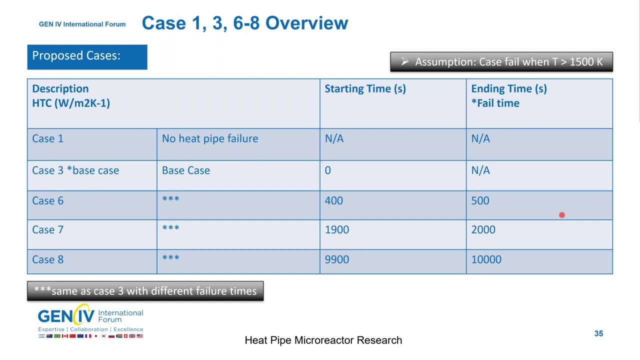 from all the heat pipe, no matter it's from ring one, ring two or ring three. So let's look first the group of our calculation and we compared different numbers of heat pipe fails and we check the result And after that we concede what will happen. 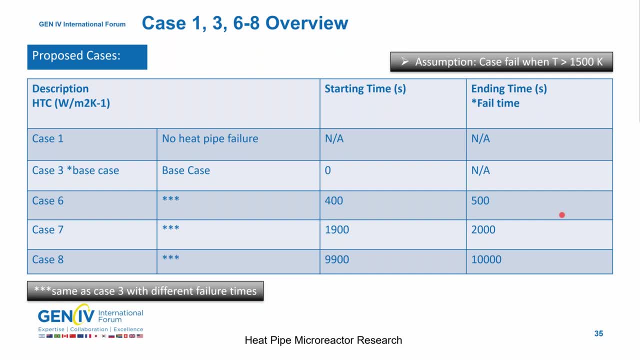 if things have, if the same heat pipe number fails but it happens at different time. So here we keep the case one steady state and we use case three as the base case. Here two ring of heat pipe fails at zero seconds. And from case six to case seven. 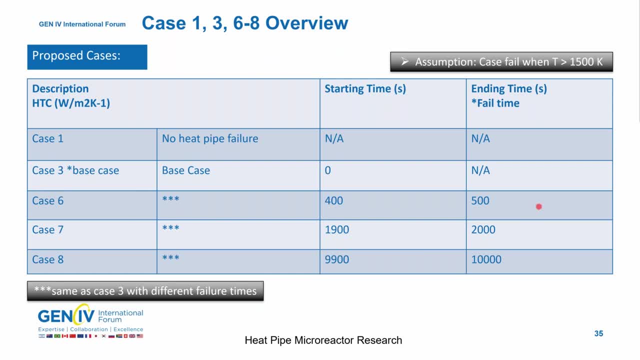 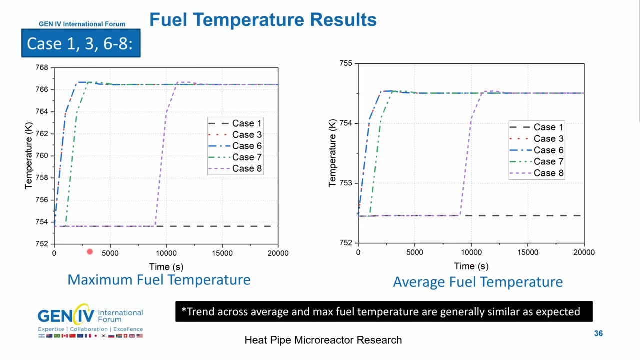 all of them are two rings of heat pipe fails, but it happened at different time: 500 seconds, 2000 seconds and 10,000 seconds, And then we will check what will happen. So here's the results. First, the result I show here: 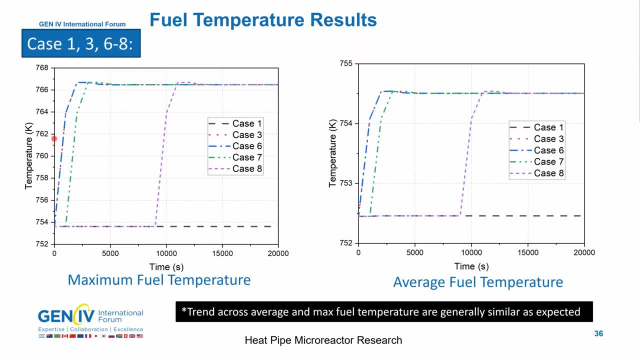 it's the maximum and average field temperature And we can find the light Case. one is the steady state And for the other case they have the same tendency that at some point the temperature were increasing because two rings of heat pipe fails and the model is. 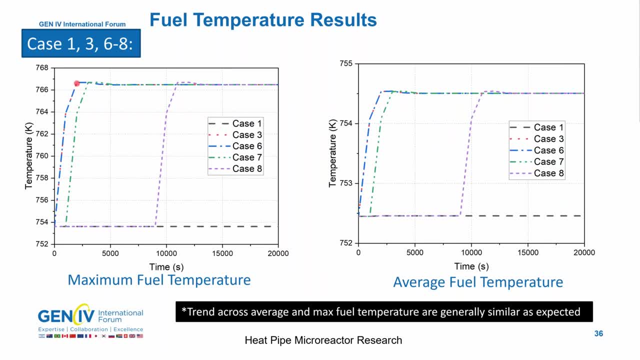 and the heat pipe are suffering a higher energy input And at some point it will comes to a state, steady state, and the peak temperature will stay here, And then the tendency for all of these case are same, but it's kind of delayed due to different. 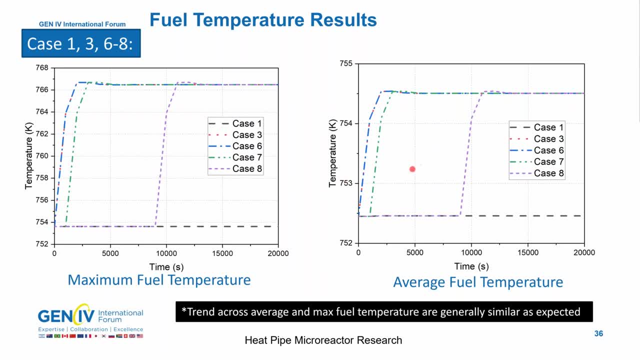 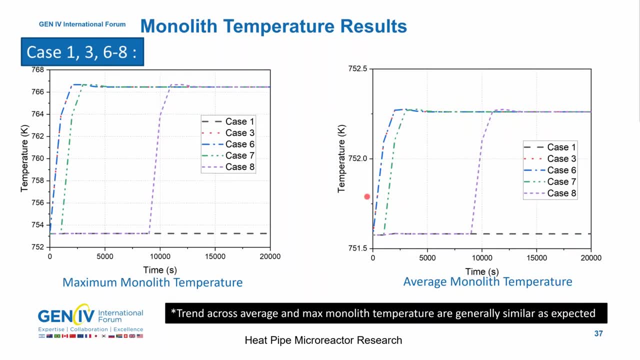 on failure time for heat pipe, And also the situation is similar for average field temperature. And then we also check the situation for the maximum and average model is temperature. Same conclusion here. All the case are kinds of delayed Depends on the different failure time of the heat pipe. 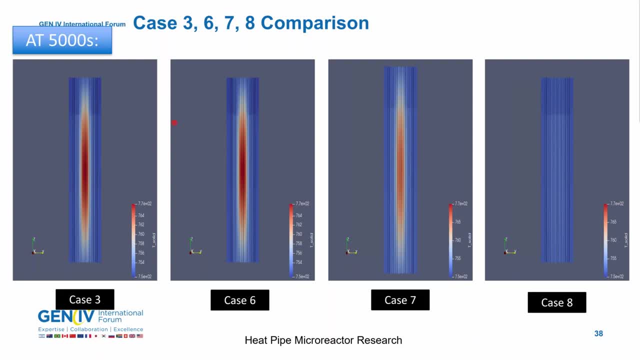 And then we compare the 2D cloud temperature of case three, six, seven, eight at 5,000 seconds. So at this point case three and case six. So case three: heat pipe fails at zero seconds. Case six: it fails at 5,000 seconds. 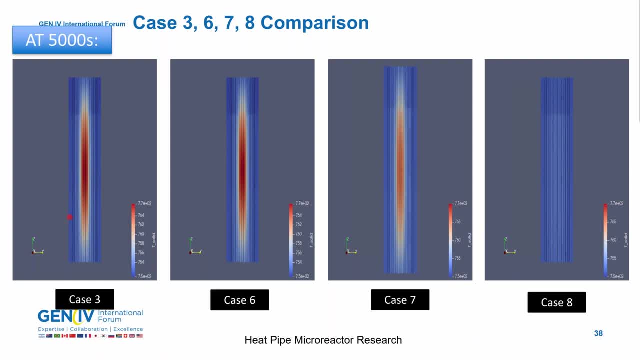 So for both of them, at 5,000 seconds, the temperature already reaches to a steady state, the peak point, And in case seven, the temperature is still increasing. And in case eight, nothing happened yet. at 5,000 seconds, 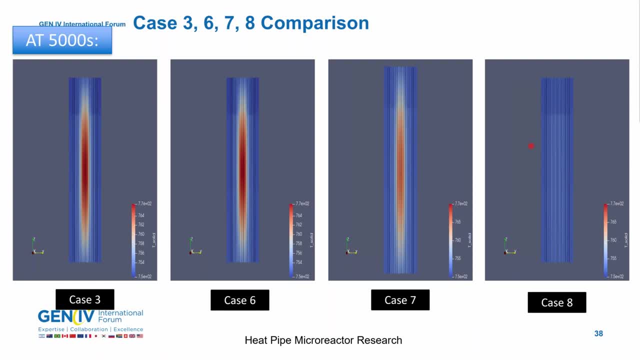 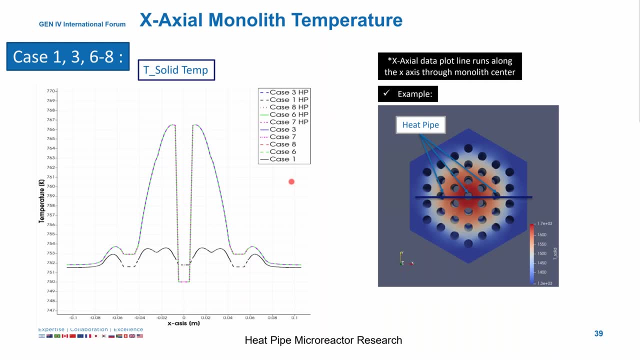 And that's why we observe a different temperature in different case And another temperature comparison at 20,000 seconds At the end of the calculation. So we have observed the tendency as DSM and for this line at x x zero And the peak point is heat pipe. 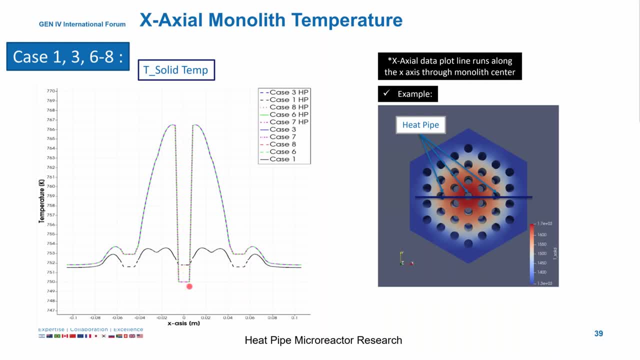 low point. heat point is fewer and the low point is heat pipe And at the end of calculation all the three case reaches to its peak temperature. So no matter how long you hold the failure of heat pipe, finally it will come to the case of heat pipe. 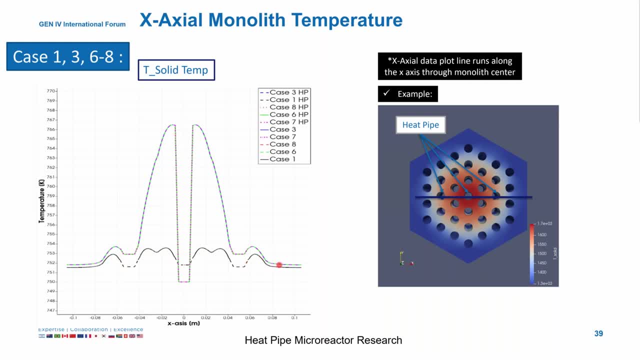 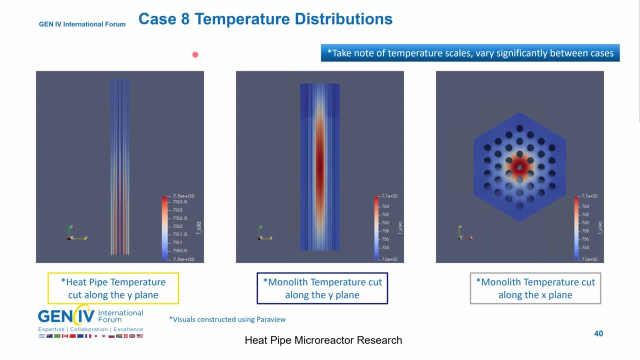 And the early black line. here is the steady state. and for the comparison- And here we selected one case, case eight, as an example to show a distribution, So here is the heat pipe. model is from side view, model is from top view. 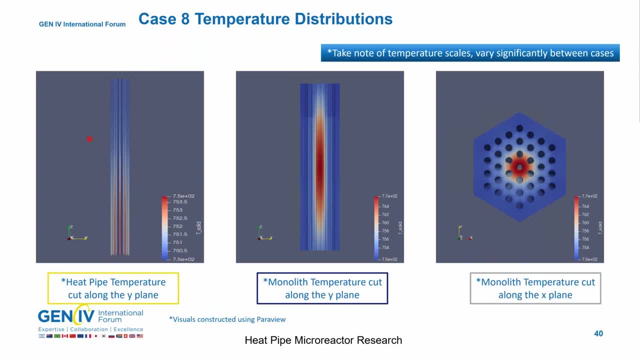 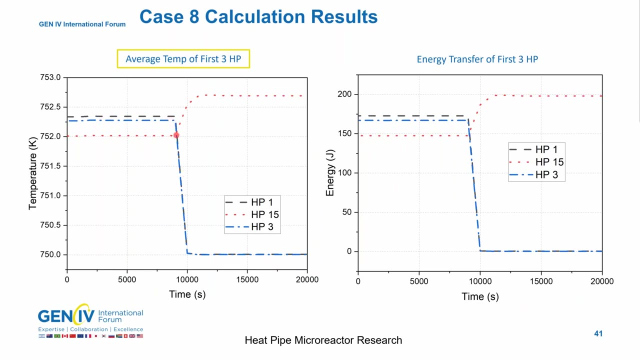 And if you still remember what I showed for case three, so at 20,000 seconds, the temperature distribution. it's then from case eight to case nine, Case three, And we can also check the situation of heat pipe. We can see that ring one and ring two fails. 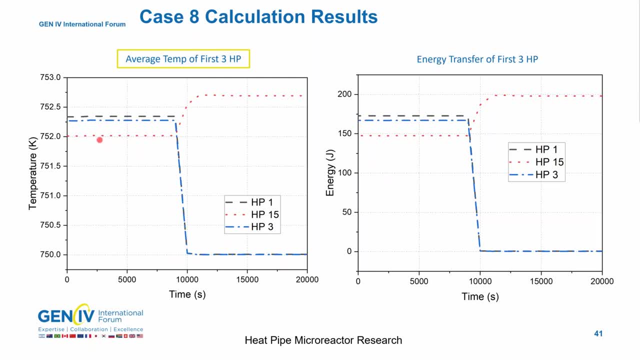 at 10,000 seconds And ring four, ring three and other rings is taking higher heighten, higher burden, And the situation is same for energy transfer system. So in this second group of our calculation we check the heat pipe. two rings of heat pipe fails. 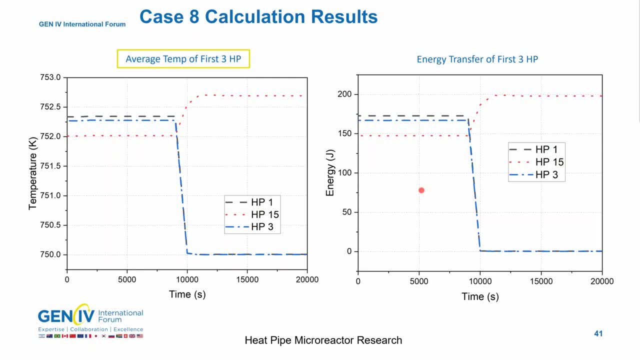 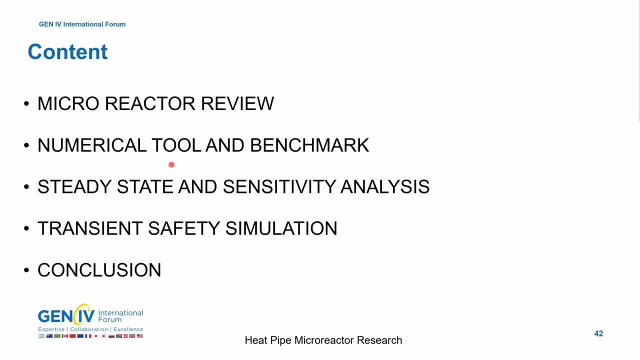 and then we get the conclusion: like, the delay of heat pipe failure won't change the tendency of changing the case, but it will be delayed due to different delay of the heat pipe failure time. And finally, based on all this calculation, no matter steady state or changing the safety calculation, 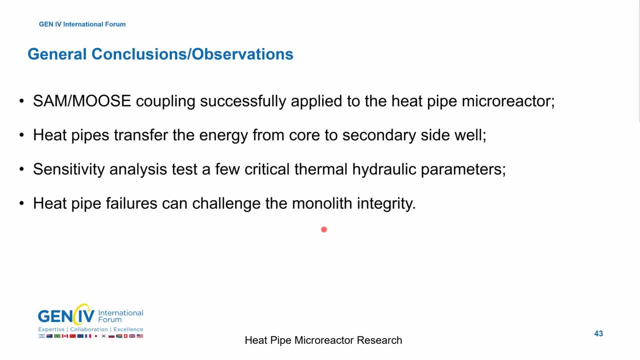 so we can see if it comes to our conclusion. So we successfully developed a 3D and 2D SAM and MOS covering system and applied it to heat pipe micro reactor And we checked that energy can be safely removed from the primary system to secondary system. 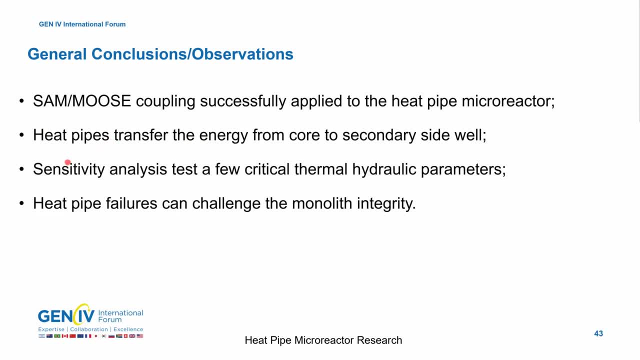 by the heat pipe technologies And we did a steady state calculation and check some critical parameters for sensitivity answers. And also we check some transient safety case to check different numbers of heat pipe failure and heat pipe fails at different time And we can get to a conclusion, like some case. 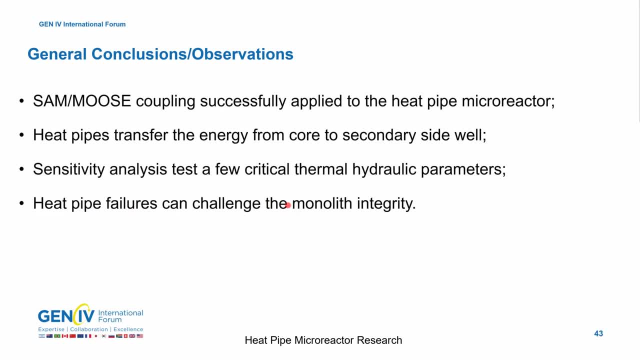 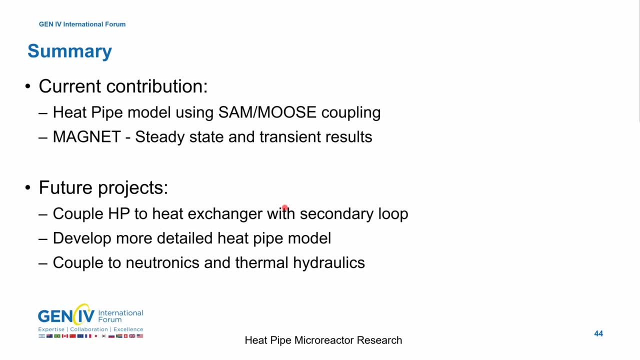 of the transient case can slated the integrity of heat pipe micro reactor system. So in the future we will work on foreign projects. First is we will build a more detailed heat pipe model based on every design, And we work on this by covering with wasting house. 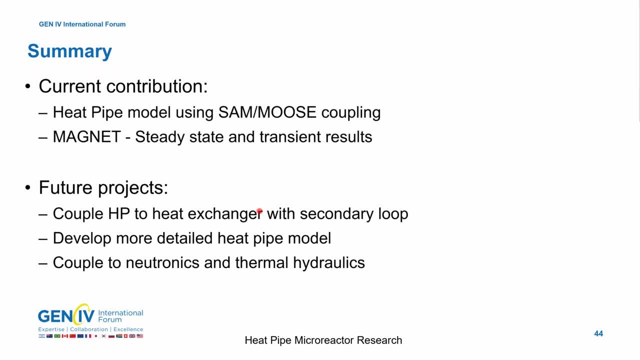 And at the same time we will develop a heat exchange technology. We might use super CO2 to transfer energy from a condenser heat pipe part to the secondary side. And all this work, we will integrate it with wasting house, every group. And another thing we can do is consider enrichment. 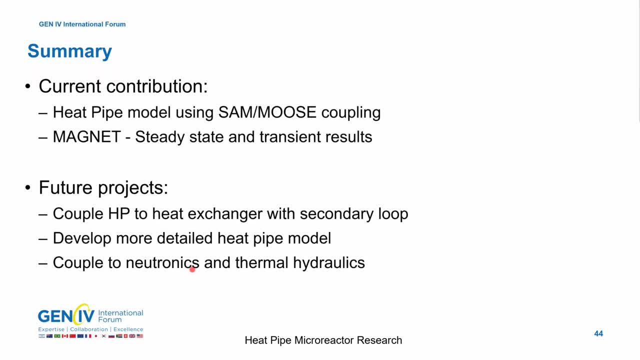 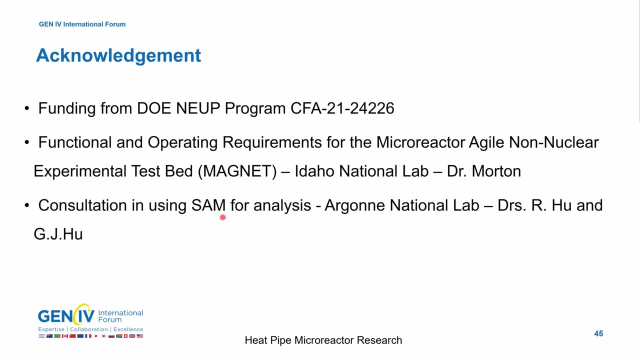 of the fuel in the heat pipe micro reactor system, coupling the neutronics and some hydronics and set the fuel into different ignition power in the calculation And at the end of our presentation I would like to thanks for the financial support. 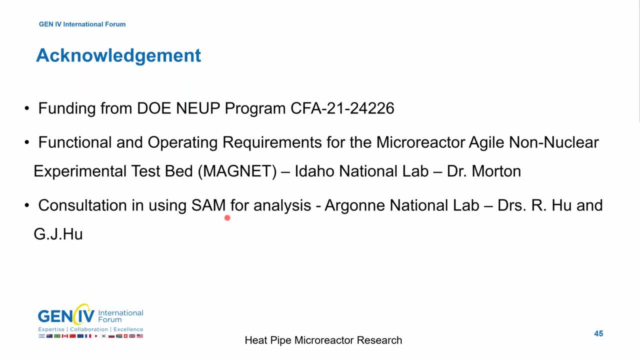 from United States Department of Energy NIAP program, And I would also like to thanks for the support from the magnet manager, Dr Morton from Idaho National Lab, and also to Dr Hoos from ARCA National Lab, the developer group of SAM software. 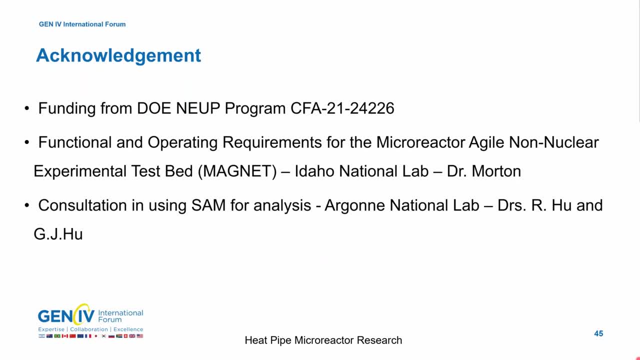 Thank you very much for your support And I also like to thanks for all the audience, patient and your time to listen to my presentation. Please let me know if you have any questions. I will be more than happy to be here to discuss the details with you. 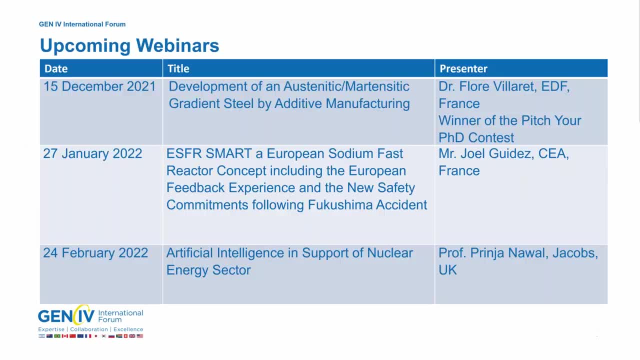 Thank you very much. Thank you. Thank you, Dr Wang. As questions are coming in, we'll just take a quick look at the upcoming webinar presentations that we have scheduled In December. development of an austenitic martensitic gradient steel by additive manufacturing. 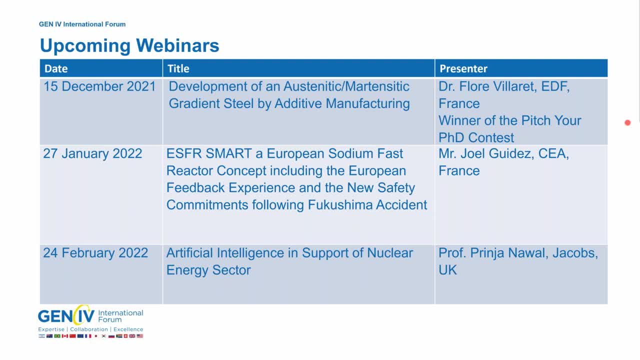 that presentation will be given by Dr Valera. She is the winner of the Pitcher PhD contest In January. ESFR smart: a European sodium fast reactor concept, including the European feedback experience and the new safety commitments following the Fukushima accident by Dr Joel. 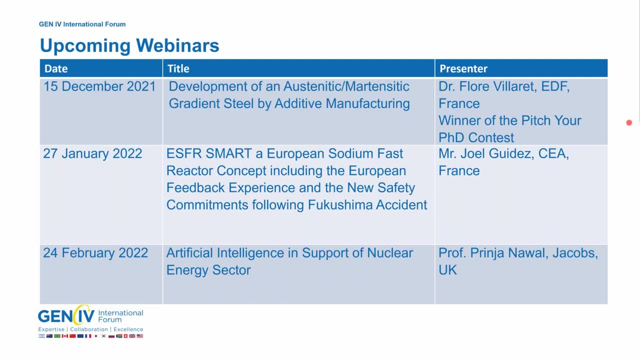 It is In February. artificial intelligence in support of nuclear energy sector by Professor Newell. We do have some questions. Let me get. let me set it so that you can see them as well. All right, So you should see a pane that has the questions listed. 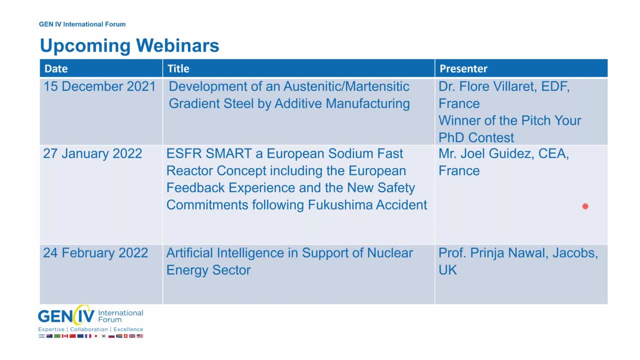 Let me get those. Okay, So, let me see, Okay. So the first question is both you and Patricia Dr Wang. The first question is: do you consider the thermal properties of vapor wick and wall constant with temperature? 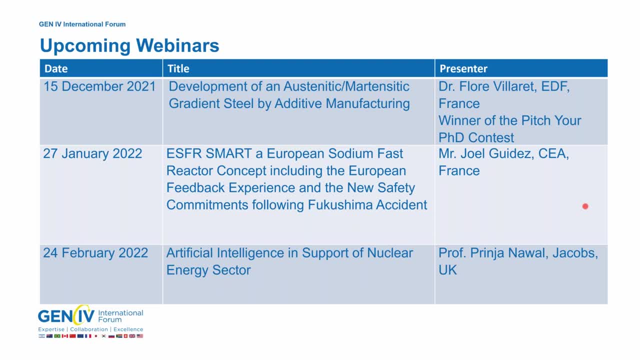 Okay, Yeah, Thanks a lot for this question. So so for sure, the vapor, the, the coolant, the temperature has to change because ignition status- oh sorry, we are asking the thermal properties. So for the weak and also for the warm, 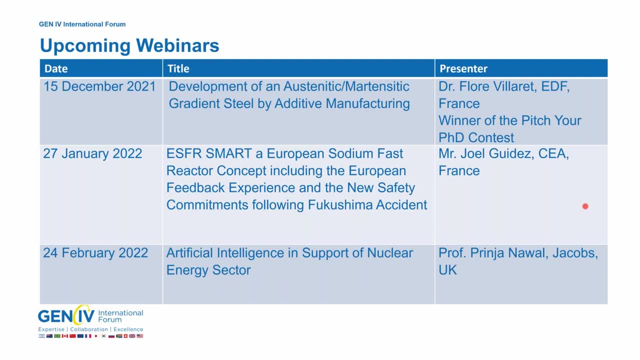 we are using the constant temperature and for the coolant we are using the constant thermal properties for the material And for the 2D sodium. I assume in the 2D heat panel model in SAM the thermal properties could be changed due to different temperature, but we have to check. 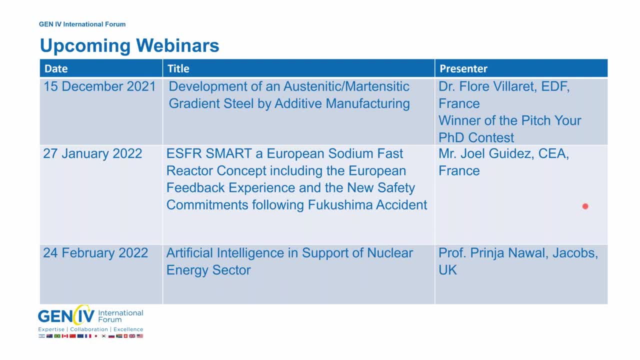 with the code developer from Argonne National Lab. Thank you. The second question was: what is the wick material? So the wick material? it could be very different from the different design. So if you want to check the details, I suggest you Google a company's name. 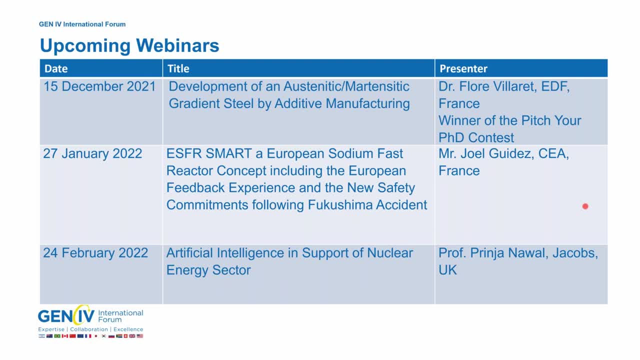 called Advanced Coolant Technology And it's specific. it's an industry supply for different types of heat pads And there are many wick materials can be considered there And in our modeling, since we are using the same material with the magnet facility from Idaho National Lab. 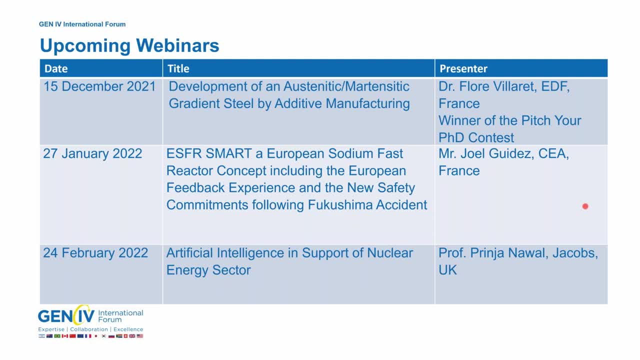 so the wick material we use here is stainless steel, but it will be very different from the reality and the industry use. Thanks, Thank you. How do you model HP and CES, The inside two-phase flow? Oh, so this. thanks a lot for this question. 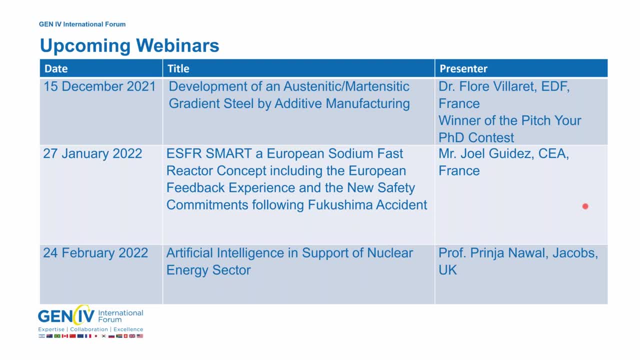 So this? so we are using a 2D heat pad model which is developed by SAM. So this work is published in SAM user's menu, which is released, And also we published a book introducing different software application in nuclear power plants. 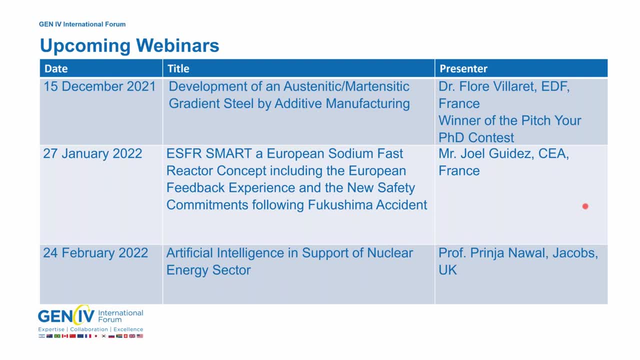 The book name is Nuclear Power Plant Software Development and Verification and Application And in one of the chapter we explain the heat transfer model in the heat pad. So it's conceived. it's separate the heat pad into nine different parts, So it's three blocks from internal to outside. 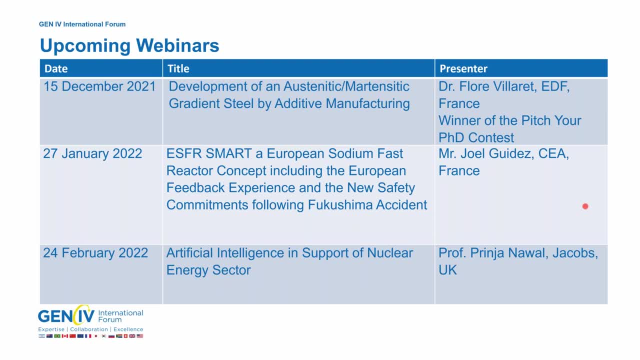 is the current weak and war From left to right. it's vapor, ideobatical and the condenser, And each in each of the block it's something like a node and there could be energy and mass transfer between each nodes. So if you want to check more details, you are more than happy to read Sam's user's menu and the book chapter Adjust the Mission. Thank you. 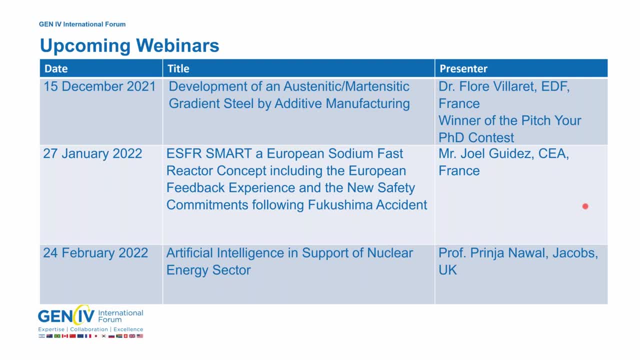 Thank you. The follow up is: can you predict HP failure due to internal two-phase flow limitation? Okay, thanks a lot for this question. So here, since SAM is a system-level calculation code, so we can see this problem and we did a transient case from the system level. 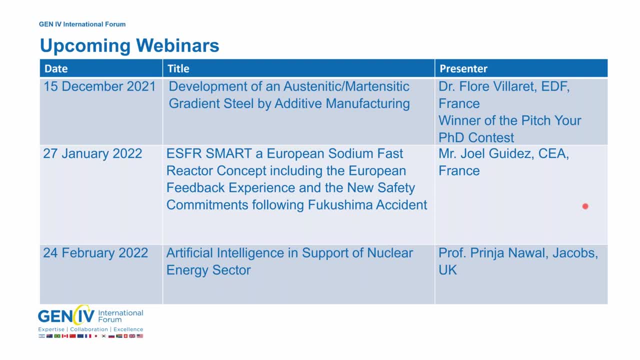 So in this calculation we directly assume HP fails and when it fails there's no heat transfer from the heat source to the heat sink. So if you want to predict and look into more details of a heat pipe of an internal model, I don't think SAM is a good option. 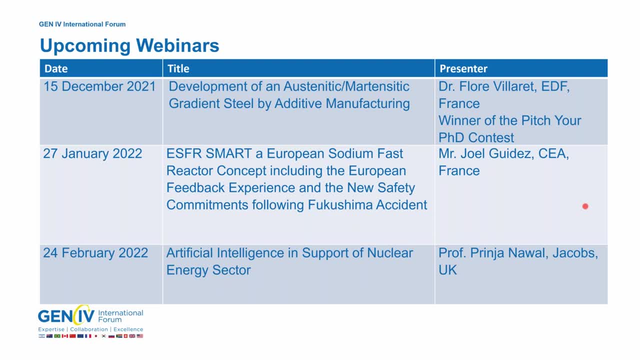 Another software I would like to suggest is SockEye. SockEye is a software originating from the Los Alamos National Lab and it's specific to look into the details, including the two-phase flow in the heat pipe. Thank you, Thank you. What would you expect the efficiency of heat pipe to be? 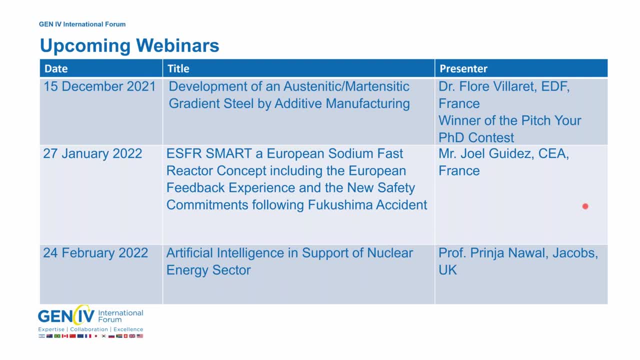 Okay, thanks for this question. So expectation at this moment is two kilowatts per heat pipe. That's the calendar suggestion and expectation And, as I mentioned, we are also making efforts to try to improve the efficiency of heat pipe. So it depends on some parameters. 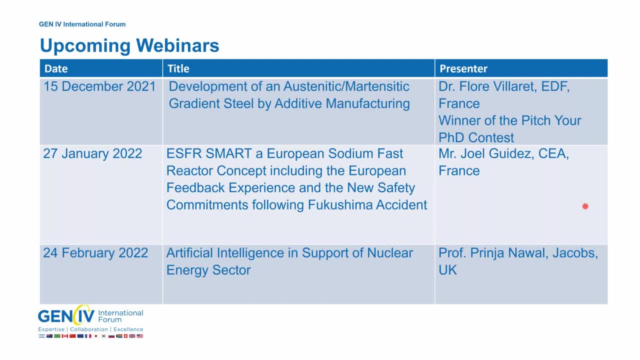 I think the most important parameter that affects the efficiency is the diameter of heat pipe. So just think that you have limited volume for current and you can increase it to a large volume So more liquid sodium could be contained in the heat pipe, So more energy could be transferred. 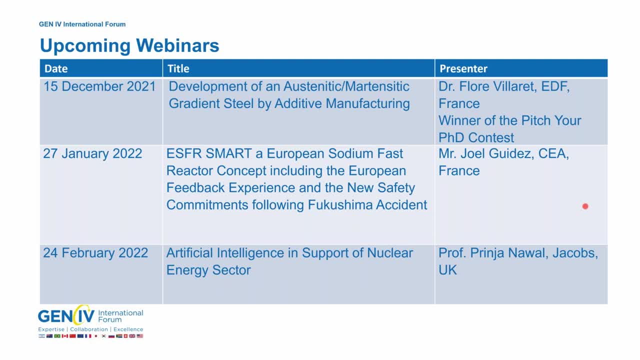 And some other parameters could be things like the thermal properties of the wick and the whorl, which decide how much energy, and the calculation speed from the primary system into the heat pipe. Thank you, Thank you, Dr Jin, did you? 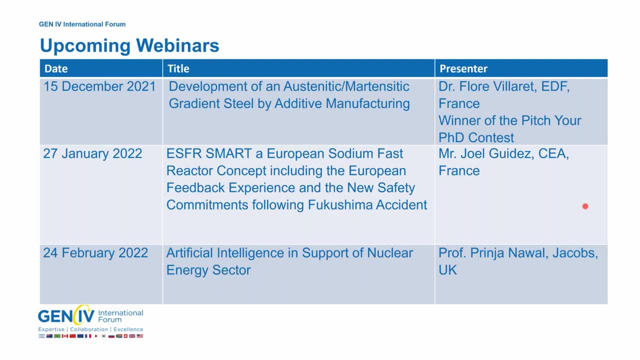 have a chance to simulate the effect of power increase on heat pipe performance power transient, And if so, this sheds light on the following: And did you model the startup or shutdown of transients? I don't know. Do you see that one? 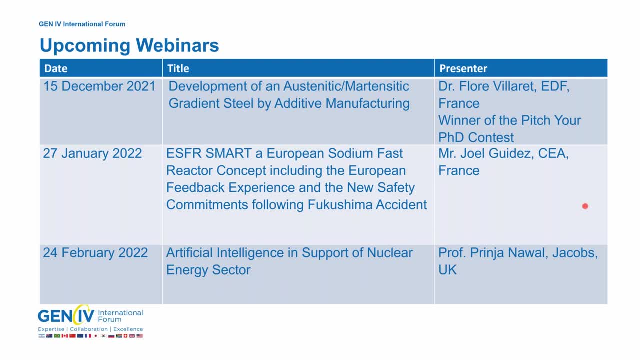 Do you want me to read it again? Oh, I'm okay, It's a long question, I'm still using it. Yeah, I was going to say Yeah. So in this calculation, as I mentioned, we focus on the system level calculation. 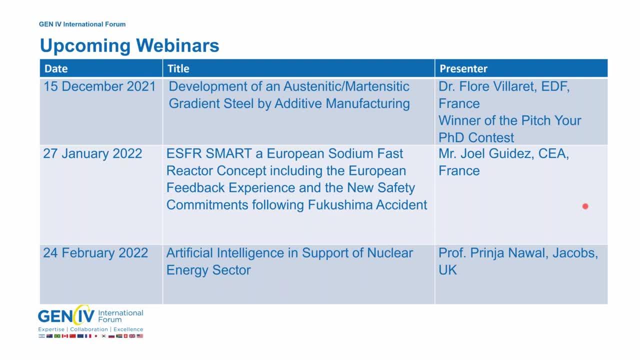 So we mostly are looking for the hot pot in the micro reactor system. So an audience asked how we can see the effects on the heat pipe performance. So the answer is we didn't consider this situation but we have some parallel project to study the heat pipe performance in the region. 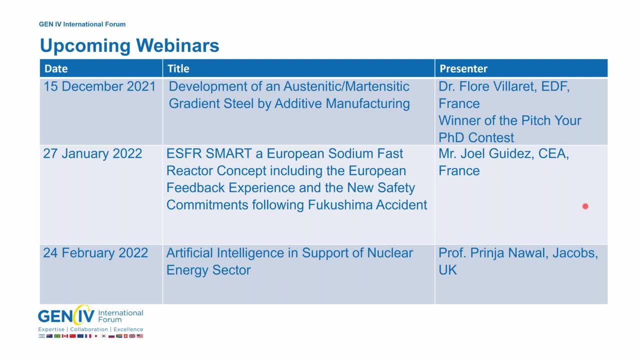 So, for example, with our collaborators from the current technology and Argonne National Lab, we are making a lifelong time performance test for the heat pipe. So which means we put heat pipe layer put into a radiance environment and change a bunch of parameters and check the situation of how it affects the situation of heat pipe. 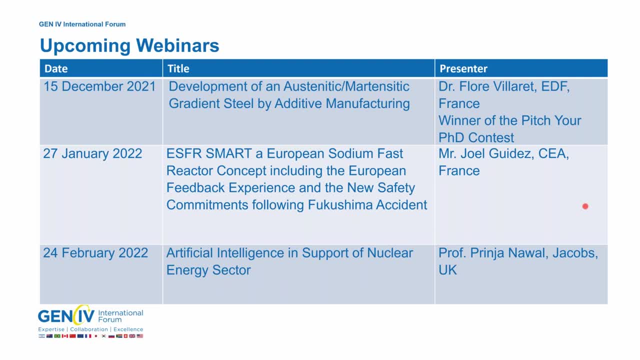 But it's not. It's not a part of the numerical work. And in my model, yes, I model the startup and the shutdown transient. So it's a very simple model, So we can see it. So, for example, for the group two calculation, we assume some of the heat pipe. it starts. 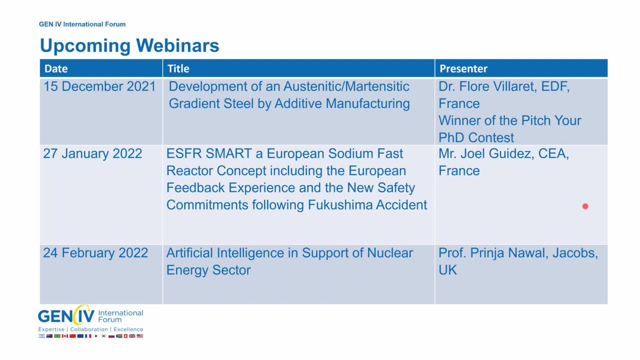 to fail at 400 seconds and then absolutely fails at 500 seconds. So there could be some linear difference of the power. So this is how we consider this startup and the shutdown transient in the calculation, But of course the real case from the experiment is much more complete. 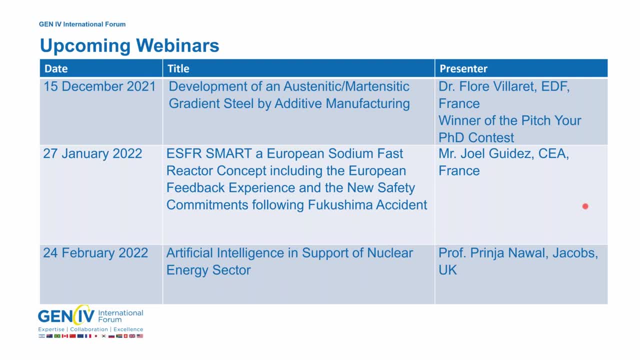 And our collaborator of the same developer is still working on another group And so both of the group in Argonne National Lab and we are still working together to improve a heat pipe model in this code. Thank you, Thank you. Do you think to consider in the future other types of heat pipes and fluids different from? 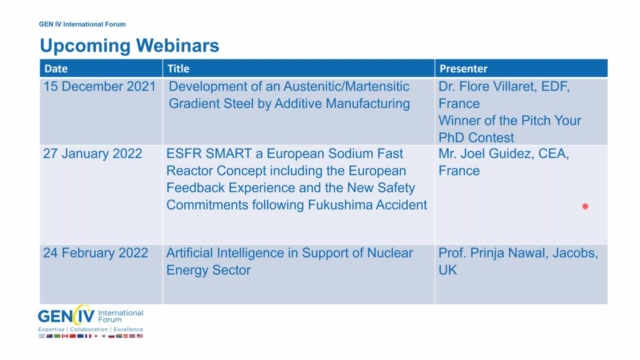 sodium. Yeah, sure, So there are many fluids could be used. So of course we can use light water in the heat pipe and the sodium, And we can also use some other current in the heat pipes, such as silver, And there are also some different options. 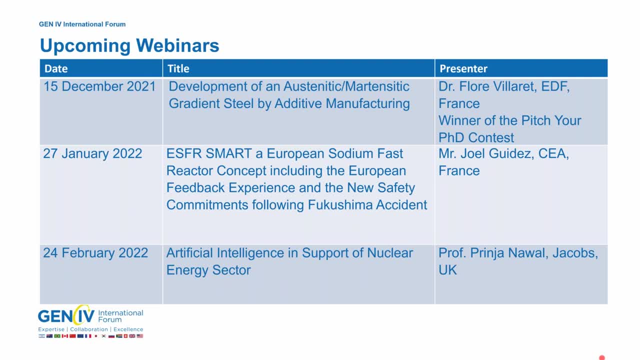 But currently we mainly focus on sodium because the sodium performance is very low And the performance can match the demand of the heat pipe microreactor And the cost of sodium is acceptable. For the other different current we also submit some proposals to trying to check and to try. 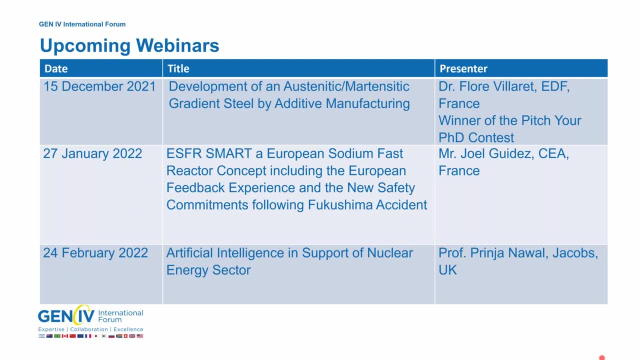 some different fluid But different materials has different limitation from the safety side, from the cost side, And, yes, we can see that We built some proposals, Thank you. So we're very excited about the future and we look forward to seeing what we can do in. 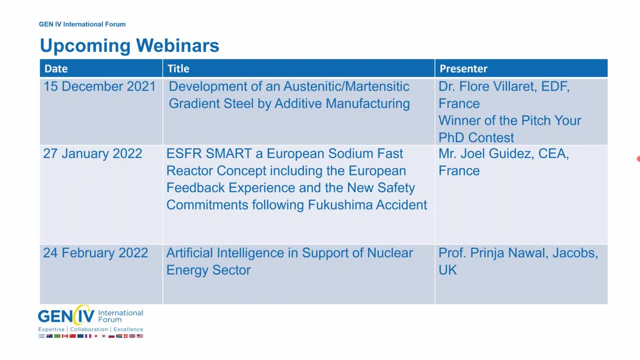 future, and then we will continue to work on the future in terms of changing the fluid. Thank you, Thank you. Will the thermal property of the base flat be considered in flat pulsating heat pipe simulation? Yes, that's a great question. 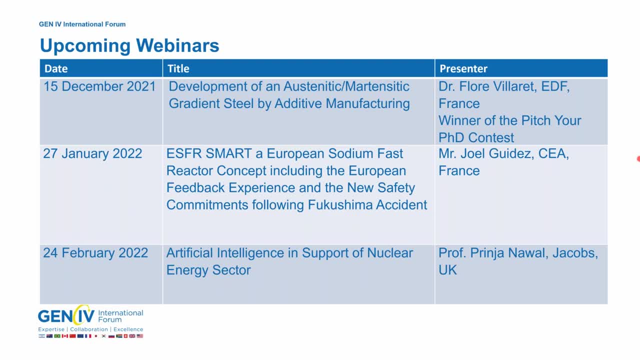 The thermal property is a little bit different. It's not necessarily a thermal property. So thanks a lot for this question. I don't think we can see it on the fried pastating in heat pipe simulation. Thank you, What is the orientation of the core heat pipes in the magnet? 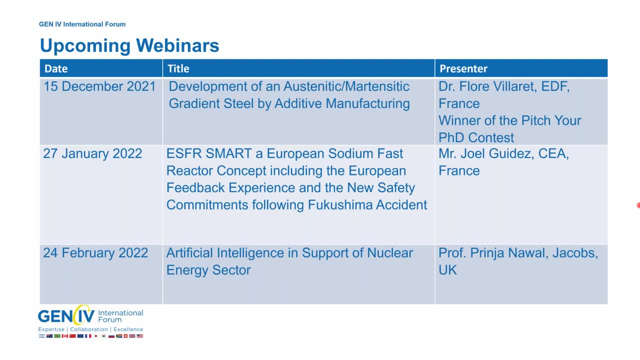 Okay, Okay, Yeah, It's, it's a very good question, Um so um, in our modeling, um, at least in our modeling, uh, currently we, we can see that it's, it's vulture. 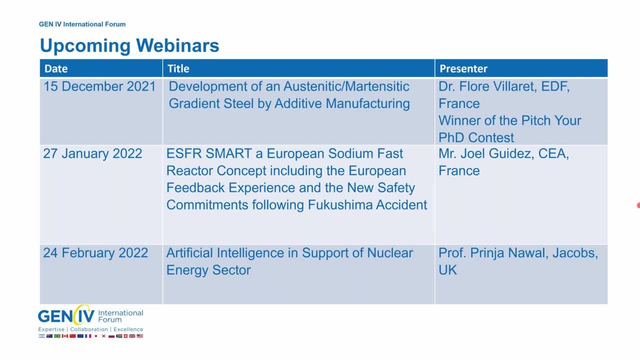 Um and remember that. so different from um, the, the, um, the other different types of reactors, such as cooled by water, Water meter. So this heat pipe micro reactor reactor core is a solid structure. So and furious storage, moderately solid and heat pipe. 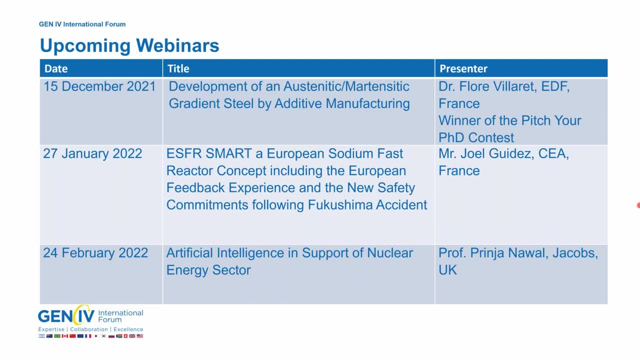 You can. you can also concede it's it's I mean outside, it's it's also cancer for, sorry, the components. So, um, I don't think The our retention of the core or heat pipes, we are fix the results too much, but I think it's a good point. 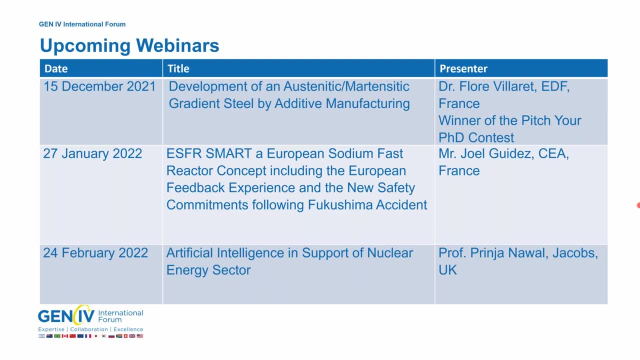 we can. we can check that in the future, thank you. thank you. what would the state-of-the-art efficiency on the electricity generation side? how mature are different kinds of TEG technologies and what would you recommend? thermal property so the different the TEG on. so it depends on heat transfer. 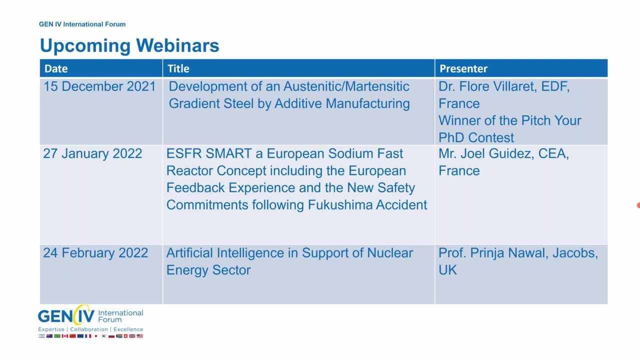 coefficient. so in yeah, I don't have too much study on the TEG technology, but I know the heat transfer coefficient should be from 10% to 15% for this technology And of course the higher the better, And also for the TEG technology, one of the most important thing. 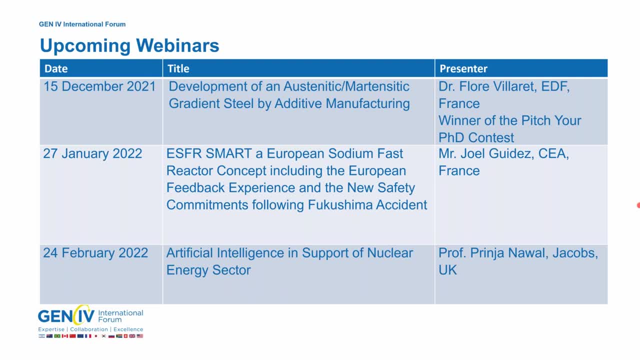 is trying to reduce the voice and trying to keep the voice in a low limit, And that's two important parameters. One is heat transfer coefficient, the other one is the voice. Thank you, Thank you. Can you comment on the heat pipe response, with increasing number of rings failed? 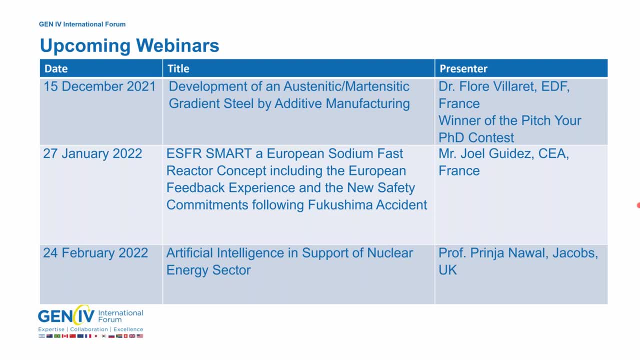 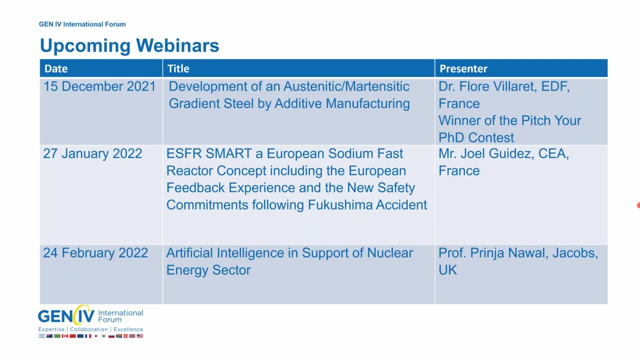 point and then slate the integrity of the system, And so at this moment, as we already discussed, the calculation is based on experimental facility. So a lot of materials such as: So it's still different from reality. Next step: we were working with Westinghouse group and using 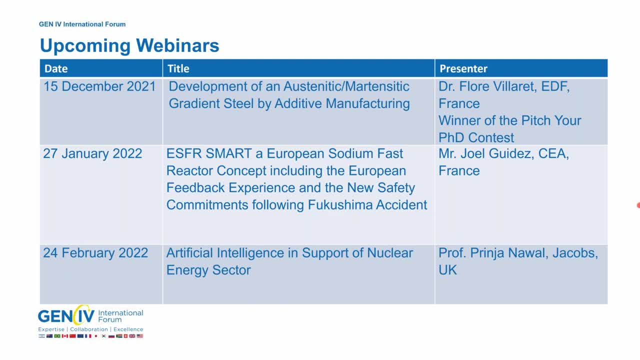 uranium and we will use graphite for the monoliths and then we will check. I think some results closer to industry And at that point I think we can reduce the risk to respond to this question. Thank you, Thank you. 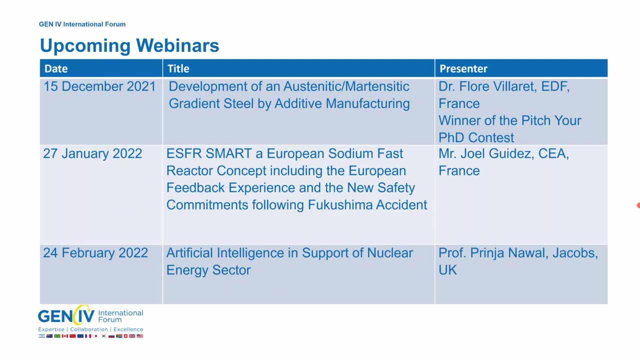 Are there welds in heat pipes that might be failure points? I don't have an answer to this question, but we have experts in our campus. That means Professor Mark Henderson. I think he will know if there could be any welds much better. 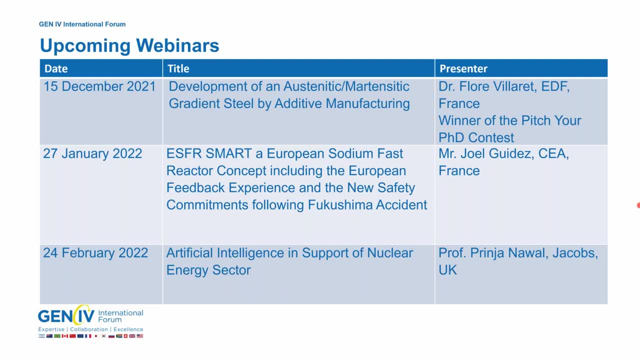 Thank you. Yeah, you can Google Mark Henderson and UW-Madison And he will be kind to give comments to this question. We appreciate your time and sharing your expertise with us. Dr Wang, Very interesting presentation of your research. That's all the questions that have come in at this point. 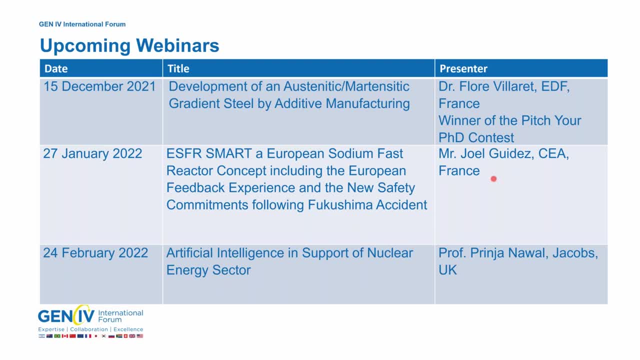 Thank you to the audience for having such a lively and engaging question and answer period. It's always impressive to see this kind of enthusiastic response to the presentations and I really appreciate your engagement. Hopefully, the system is set up to launch a survey after this webinar presentation. 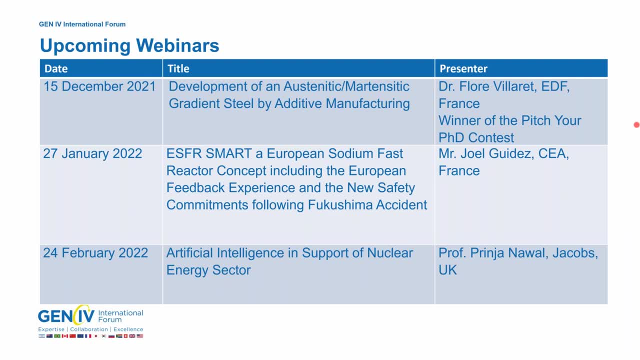 It'll be the first time I've tried this, so I appreciate your feedback and I appreciate everyone's attendance. Patricia, do you have anything to add before we close the session? No, I don't. I don't have anything to add, but again I would like to thank Professor Wang for giving a great 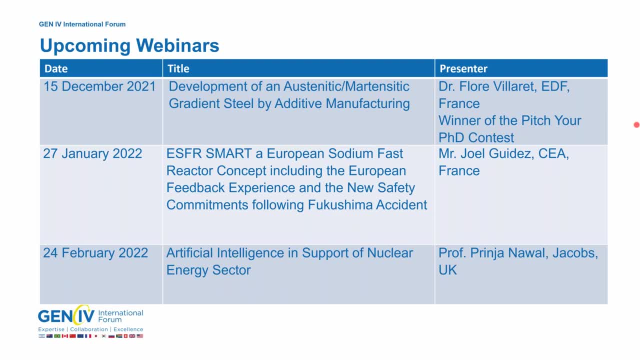 webinar. As always, it's so interesting the Q&A session, So thank you so much for taking the time to ask questions and thank you, Professor Wang, for answering those questions. Indeed, Yeah, thank you. I also would like to thank you for the invitation and also thanks for all audience patients and all the people who are here today.